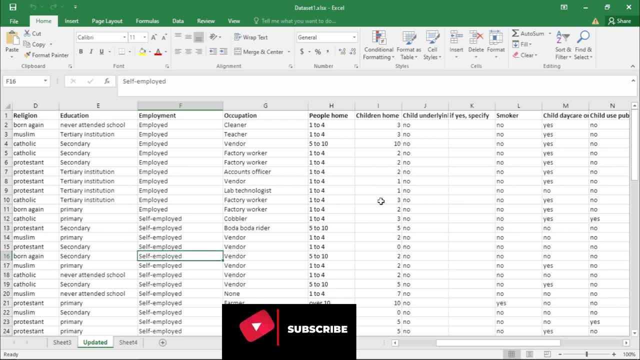 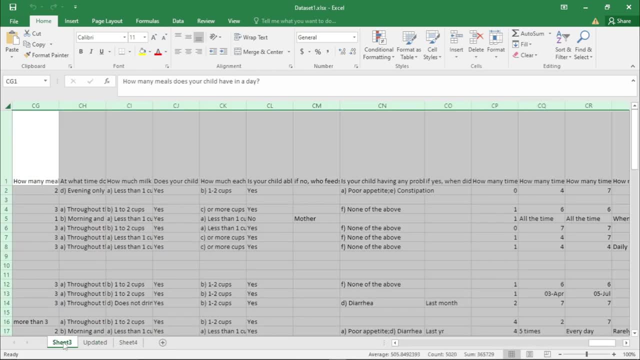 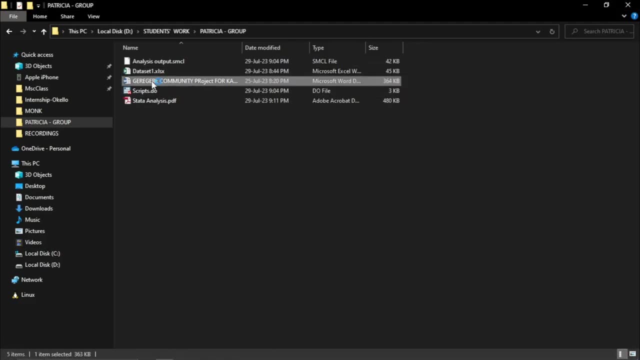 if I, if I create a database, I'll upload this. then I put the link in the description if you want to. but you can use any data set you have now. the client gave me this data set like it was that heavy. let me open the original document and I show you what the study was about, what the 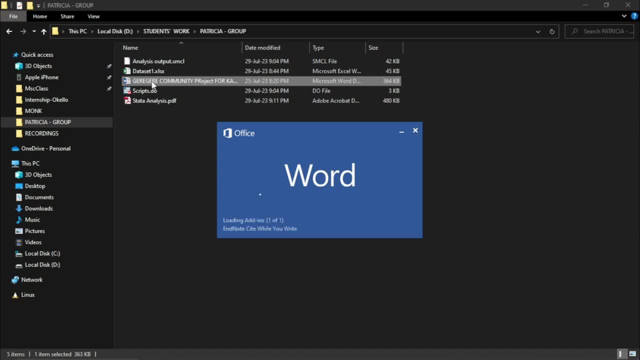 research was about, so that you have a clear idea of what we are dealing with in this case. so it may be your research. maybe, if you're collecting your data, it could be having your data available or you're about to get data set. so these are the things you will go through. these are: 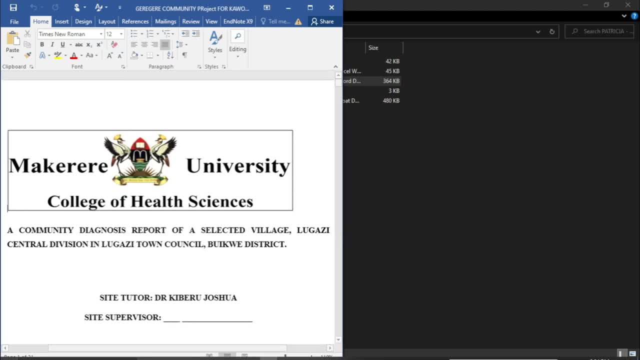 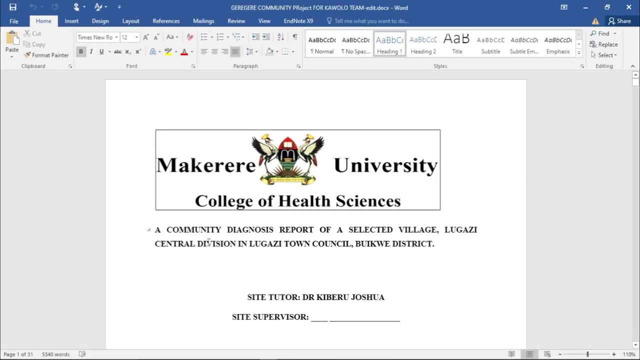 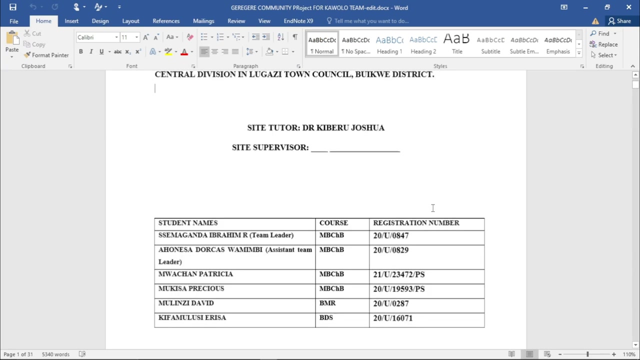 the following questions you need to be asking yourself now. so, if I look in here um this, the title for this project was community diagnosis report of a selected village, so generally it was a survey. this was being done by students doing medicine and so, uh, we are sub. 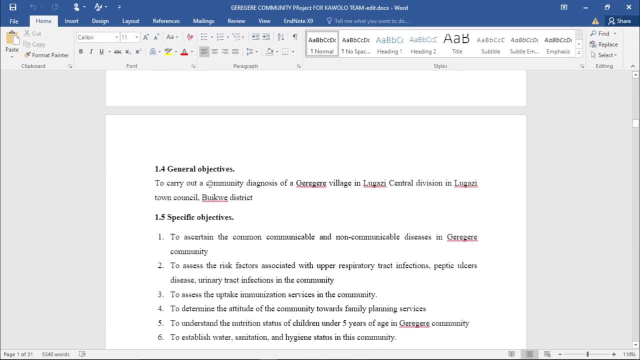 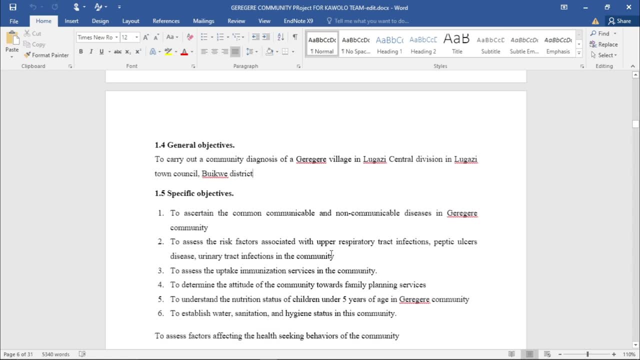 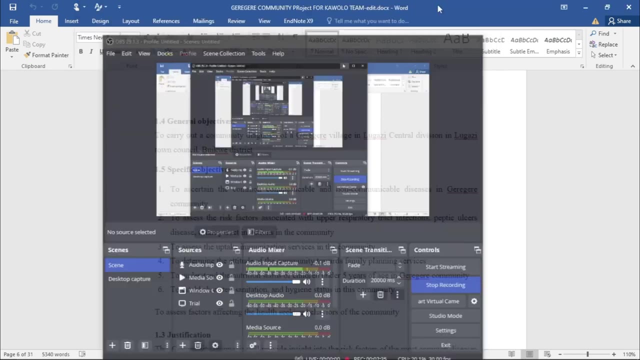 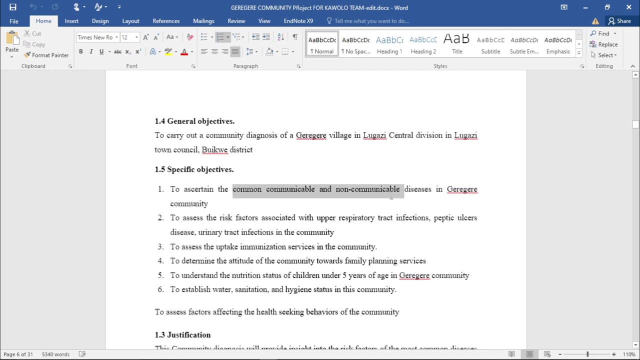 they they're supposed to go to community- try to carry out a community diagnosis just generally to find what are the the most common challenges health-wise the community people are facing now. their original objective was really broad, like they had so many objectives. they wanted to assess communal and non-communicable diseases. risk factors associated with the respiratory tract. 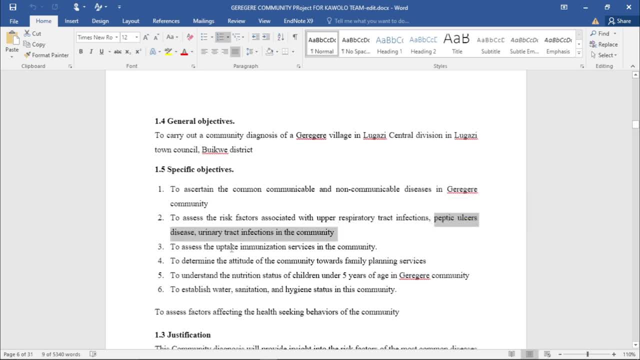 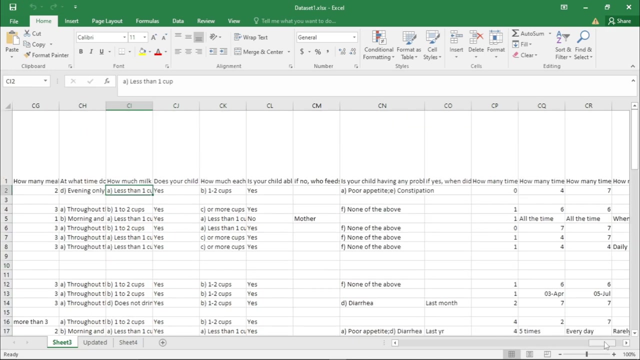 infections- peptic ulcers, urinary tract infections, among others- immunization, uptake, attitude of community towards family planning and nutrition status of children, and then establishing sanitation, water and hygiene status. this was the original idea and what they collected- this was a raw data set they really collected and this this was in excel. 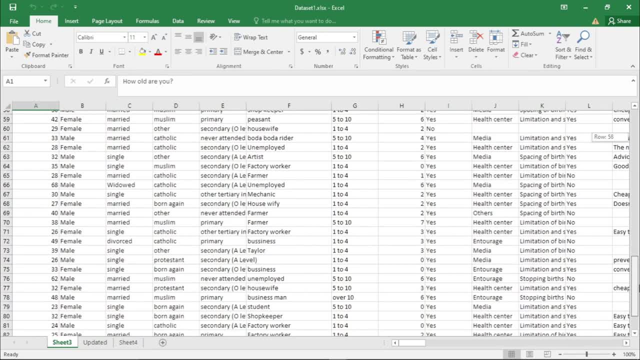 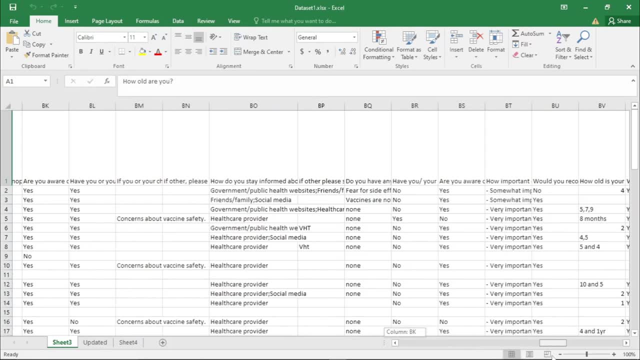 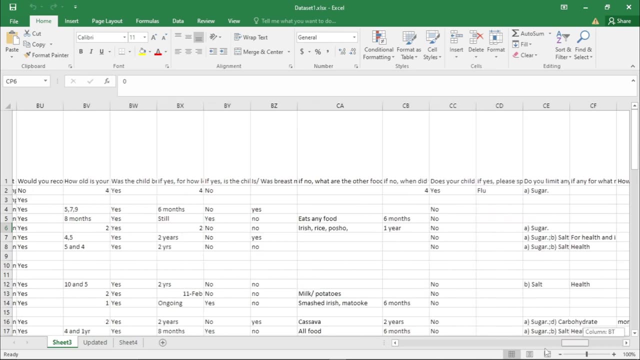 format, so it was really broad. they had all these interviews- total of 86- and then all these questions were asked and the responses were given. in total this had about 99 columns. that was collected as raw data and so they just gave her like here it is. 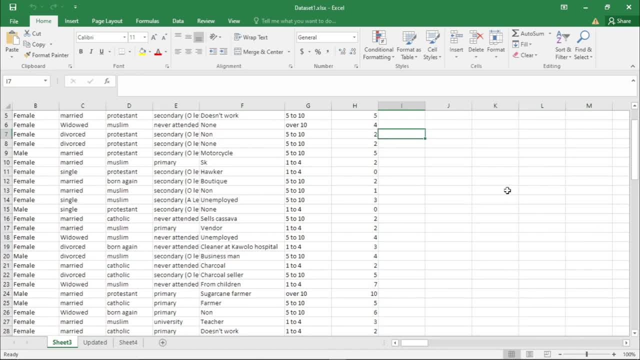 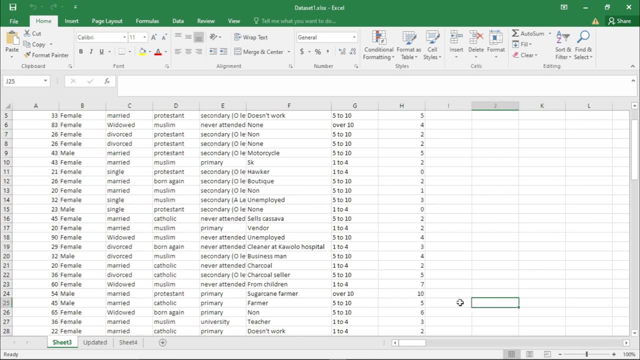 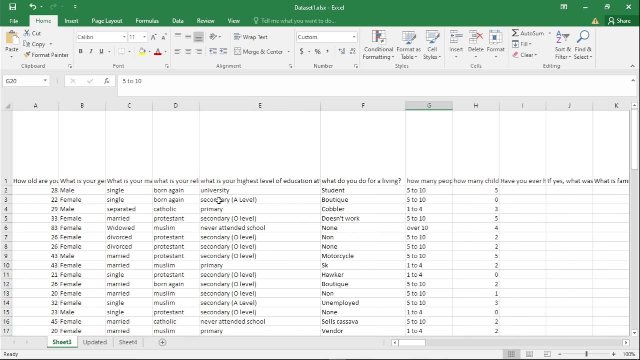 it was up to me. now, if and if you look at this road data, it had so many issues associated with it, so many errors associated with it. um, okay, others, i corrected it already, but you, you have some redundant information. for example, this was education level, now you have university. 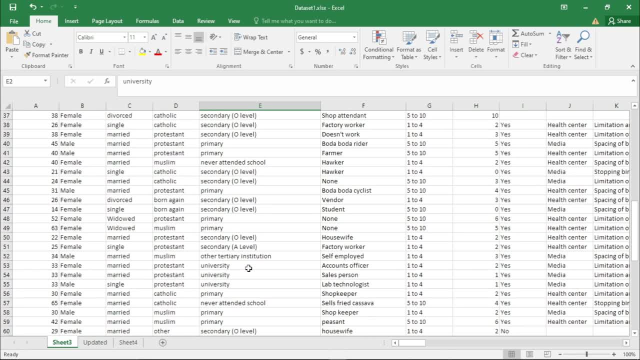 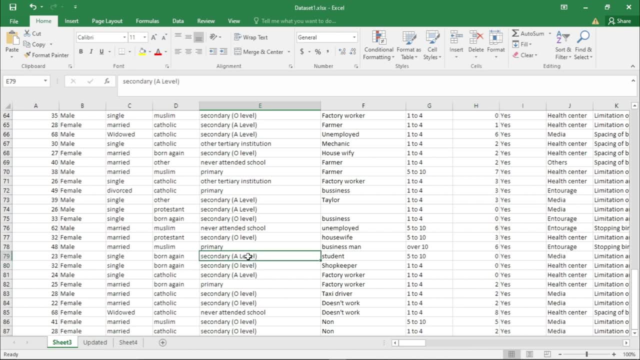 and then somewhere you have, uh, where elementary level a all right, yeah, but what i'm saying is, when you look at ie a level, is that okay, uh, secondary, or level secondary, a level that's within a similar category, university, then others you have other tertiary institution. never attended school, primary, second, 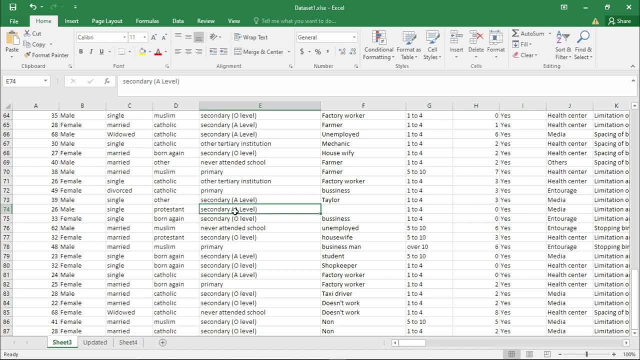 like there are so many subcategories, we could group touch rate together with the university's all at the same time. the secondary or an a level- all that is secondary level of education can also are groups you have the, the more you can have results that make sense and you can explain. 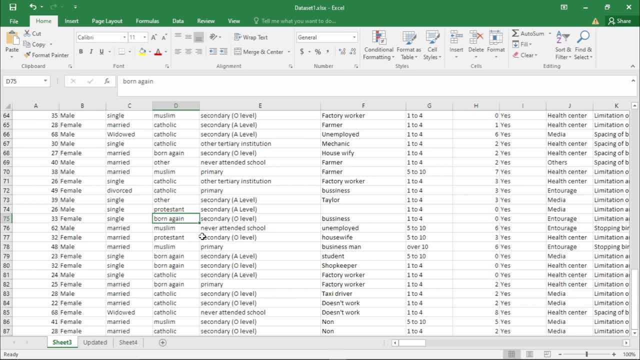 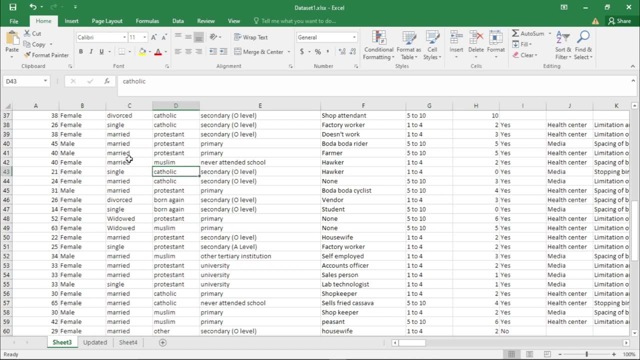 them. if you have so many groups that are like like cross divided, it becomes tough and also it depends on what you are dealing with. if you're doing a survey and unlike making all these excess groups are not going to be very, very important, in the output there is the fewer groups you have the data. 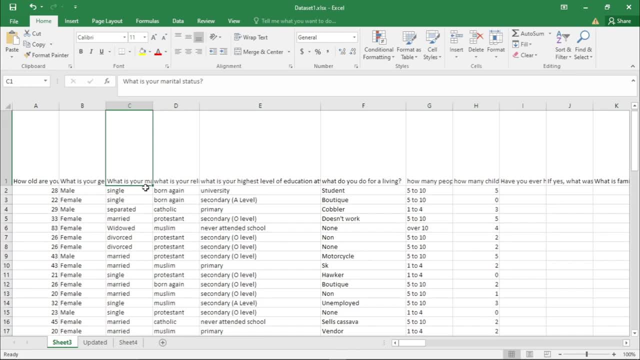 now you look at this example here. this is a marital status. so you have single, separated, married, widowed, divorced, now single. somebody who is separated is is single. somebody who is divorced has also remained single. somebody who is widowed, as has also remained single. so let's say this: you 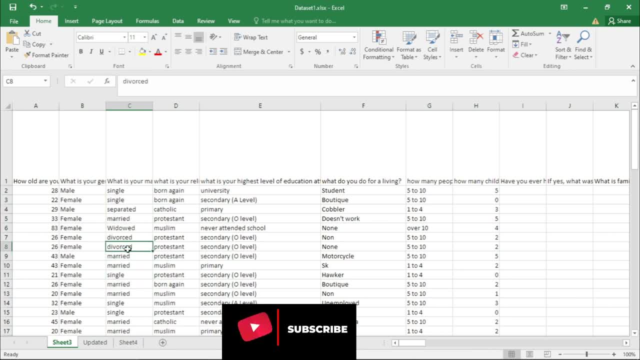 could even regroup it into married single we. it's not important for us to go deep into the details of single. what single did not marry? or single we do single divorce as long as like. does that information give us any important context as far as community diagnosis is concerned? 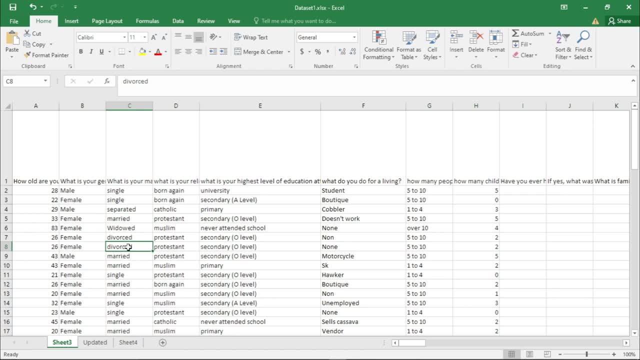 is it that important in relation to community health? no, it's not. unless we're dealing with some, let's say, hiv kind of thing, then you want to know: okay, hiv prevalence among, is the single versus the marriage, versus divorce? it is maybe, but but if it's not, then it's better to really 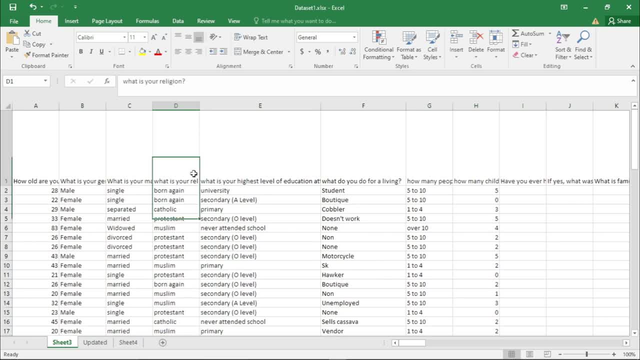 group, group group, some of some of them up, uh, things like religion. instead of having muslims, protestants, catholic, born again, others, i could have christianity, muslim, or then i add another most common group, so that you have fewer, fewer categories and you're able to really have this. 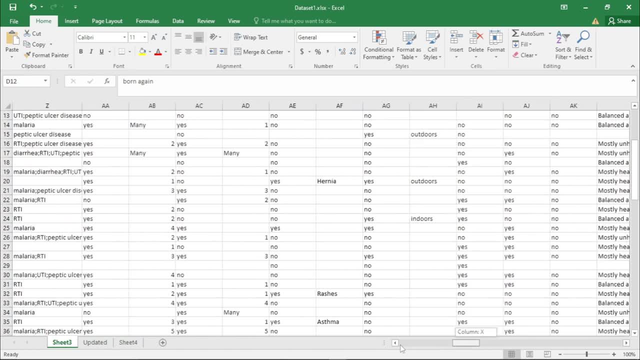 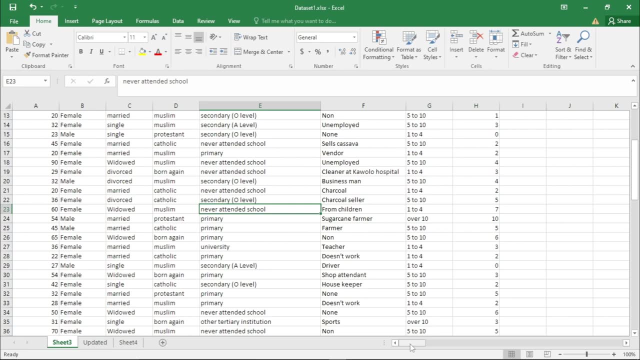 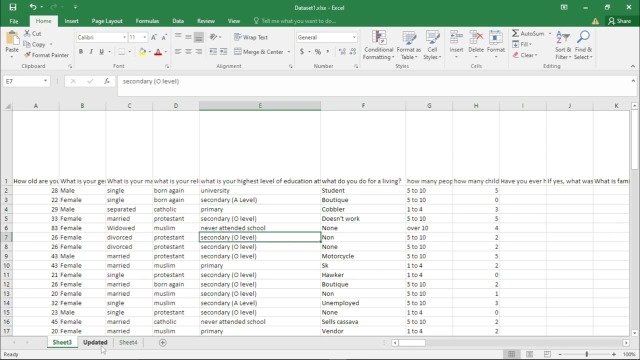 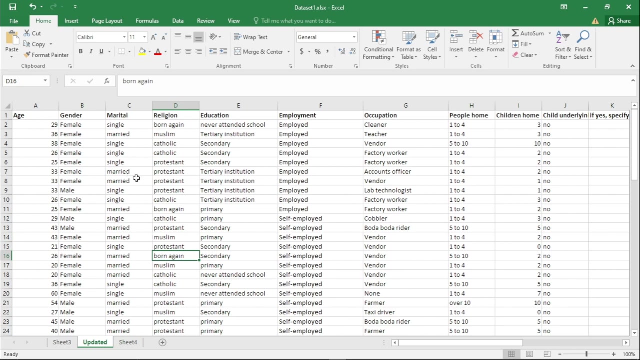 explanation in here. so, um then i mean, so this is what you'll always face and some of some of you students, or some of the students that will give you that work, they will be having this redundant information in there. so talk to them, they can regroup it. so what did they do i? i, i cleaned it up. i cleaned it up. like to really have these fewer. 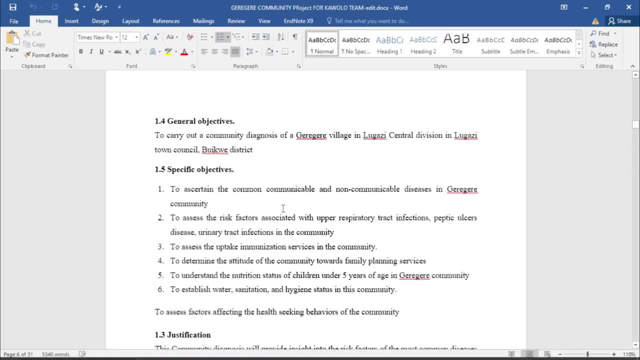 groups as much as possible. and also on talking with the supervisor. the supervisor, and because these are so many objectives, their supervisor, advised them to only stick with this, this objective to assess the risk, the risk factors associated with the upper respiratory tract infection. only. the supervisor removed everything, including this. peptic ulcers disease unit track. 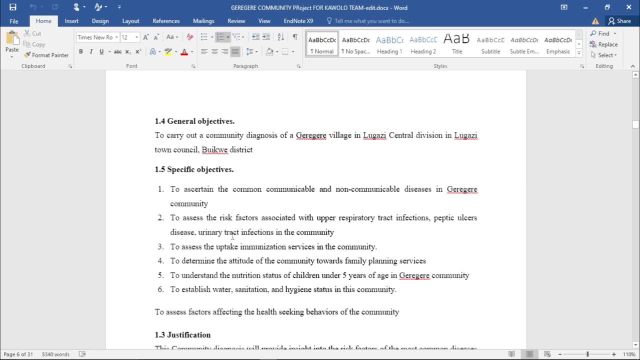 infections and etc. this was like too broad, so you may be having a study related in that category, whether social science, whether in any category. you could be dealing with factors associated with the stress among these workers working in a given bank or factors associated associated with the poor nutrition among its children, or you could be having any 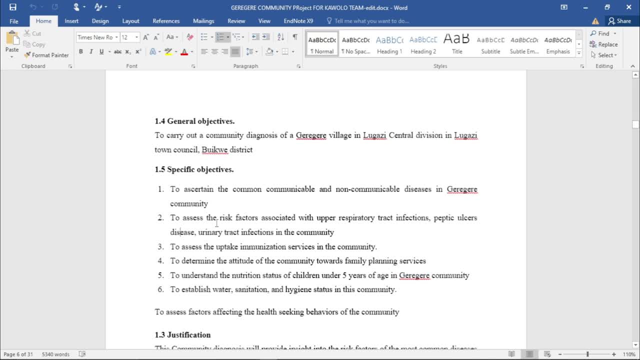 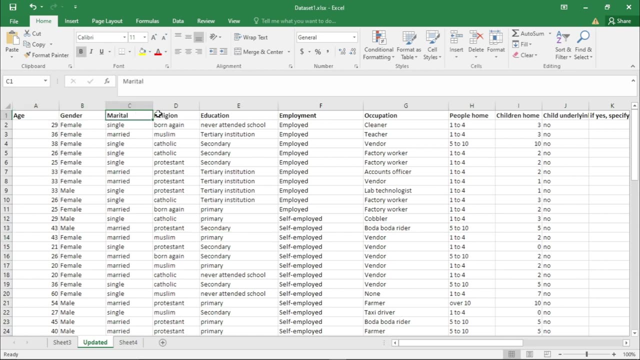 of those studies in that category, or even if in that category. so I clean this data so that I only have data set that feeds to assess the risk factors associated with the upper respiratory tract infection. this was the updated data, so only remain with the age, gender, marital status, religion, never attended. 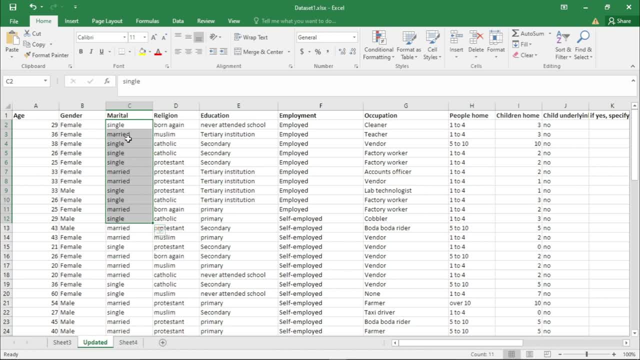 school and if you look at my two status, as I told you, I changed everything. I only remember the married single. married single. that was those are the groups I really needed. education level, all the university. I removed and combined it together to make it touch our institution, all the all and a level I. 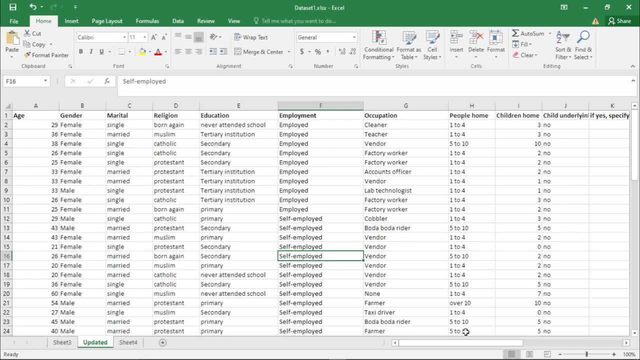 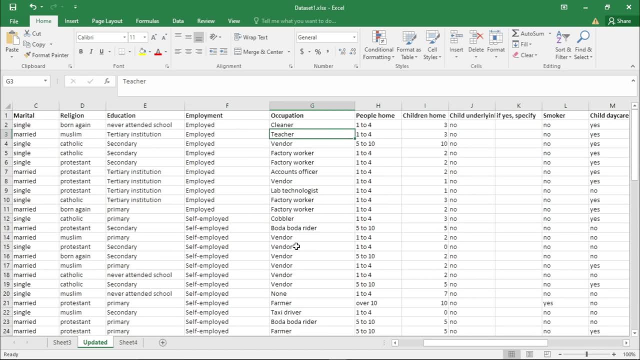 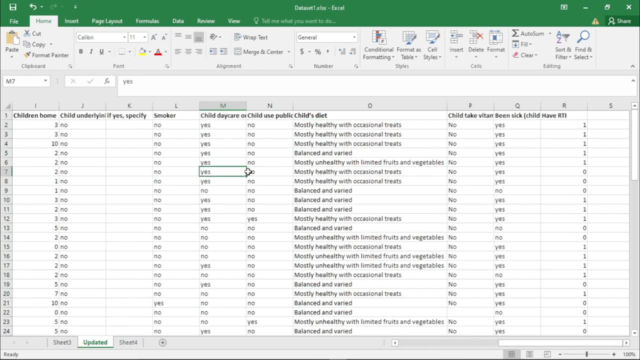 combined to make secondary education, then employment status. I also grouped them in their occupation. I adjusted it. there were so many subcategories so I also change it. number of people who are involved. over blah it is: see child's diet. I adjusted it. and then the most important part is this last one. second last question was: have you child been? 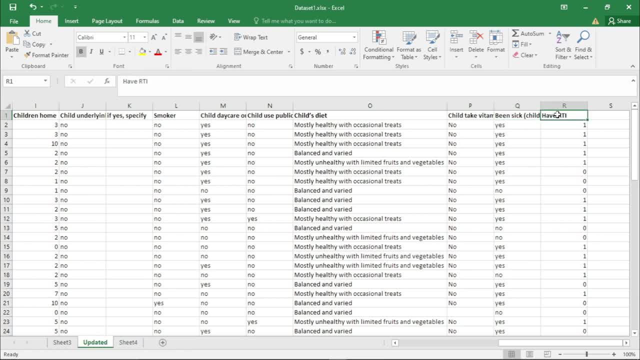 sick, then the question was: the question after that also is that: currently is your child having a respiratory tract infection? now this was recorded as yes, no, yes, no. I change it into zero. one zero, zero. zero is meaning no one is meaning yes, because our outcome of interest is. 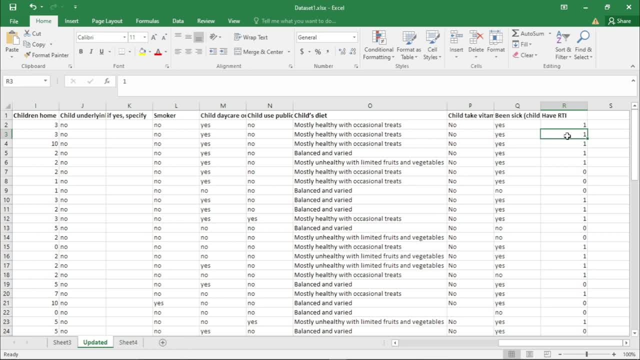 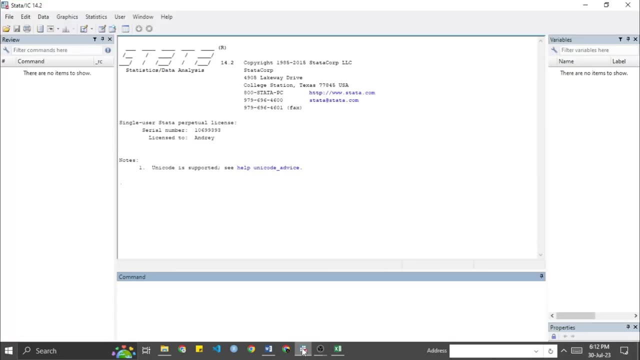 did the child have respiratory tract infection, something like that? now, when you're going to do a logistic analysis on starter, i will explain to you why this is important. now let us jump into our starter software to now analyze this data set. it's now clean and and all that. i always tend to clean it in microsoft excel. it's much more easy. 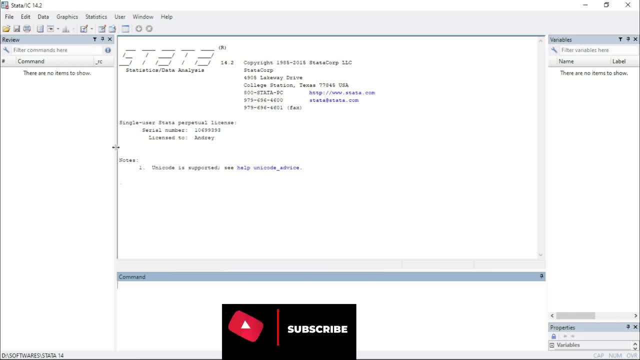 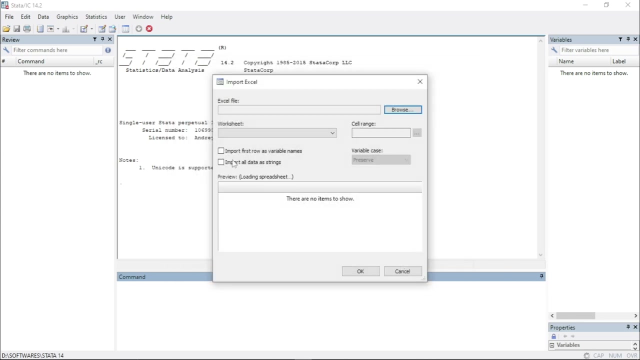 now let us import our data. so the first thing i always do if i open my starter software, i do importing, of course. so import. go to file, come to import, import excel. go to browse to choose the file. look for where your data set is open. come to the worksheet number. uh, ask yourself. 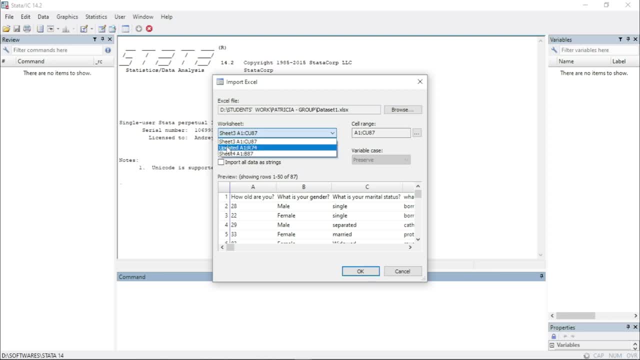 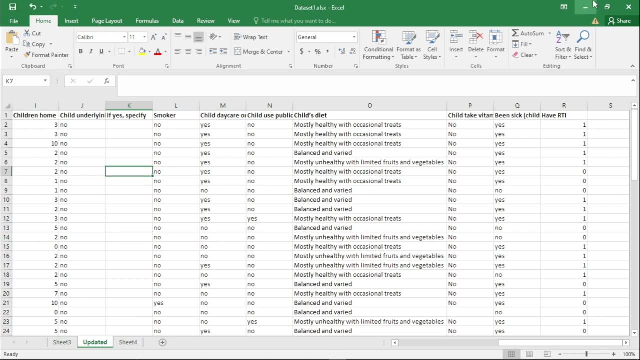 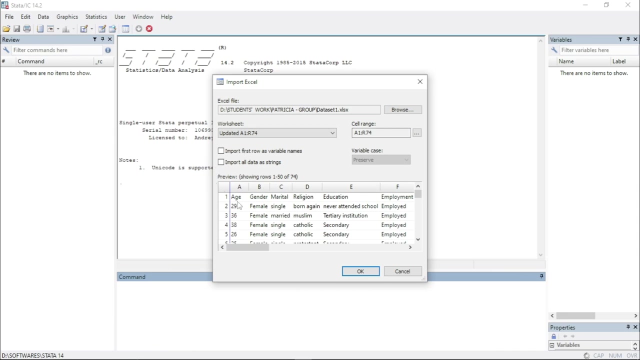 where? which position is the worksheet? this worksheet was updated, if i. if you go to excel, you see it. it is under updated. this is where the one i want, so you choose that, that worksheet. if the worksheet has only one page, there will be nothing to choose. so now, uh, it had column title. therefore, i'm going to report import first row as variable names. 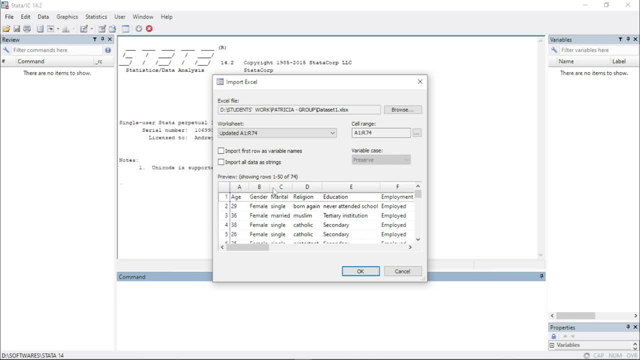 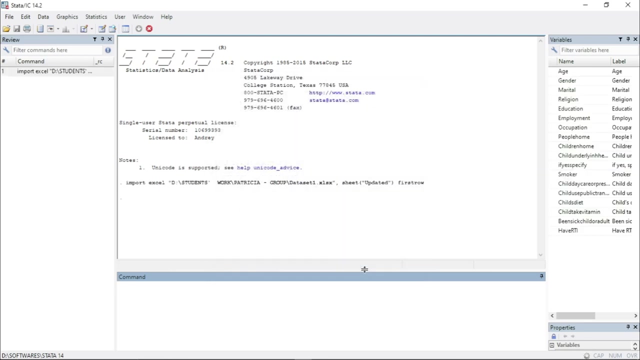 if here, if i don't click, you see my column is going to be a, b, c, d, but if i want the column title that is in my excel to be the column title in my starter software, i'm going to click import first row as variable names. so it has imported it. then i press ok. now it has opened the data set. 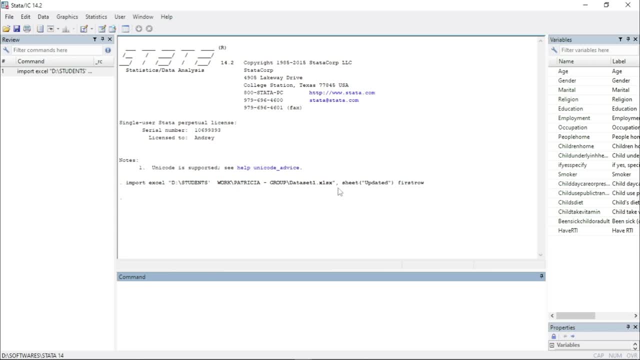 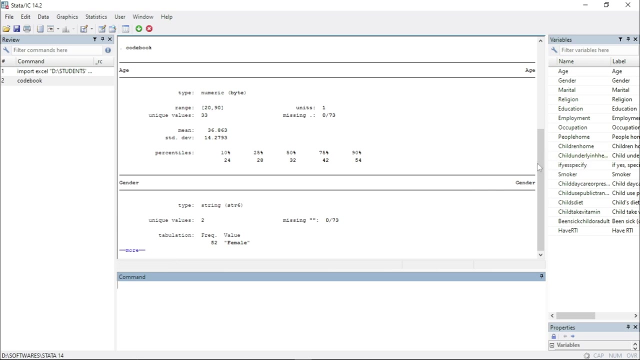 next i need to encode this data. okay, let me first check its cleanliness. so i can check its cleanness, the first thing i can do is: um, okay, uh, codebook. codebook is the first command i can use, just generally to see. it gives me a general 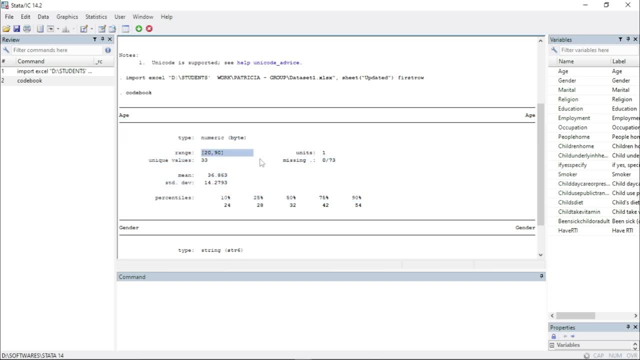 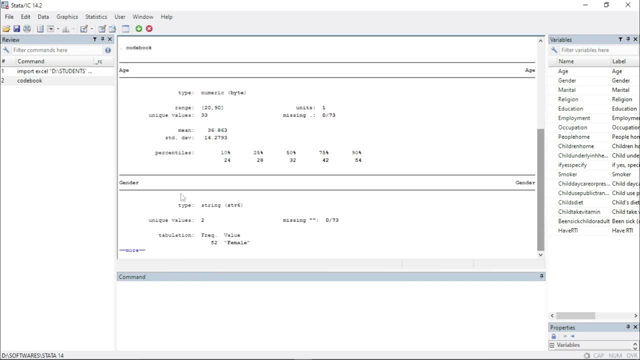 summary for one variable to another. uh, this is numeric, this is, uh, unique values are 33, the mean standard deviation. because it is numerical, then gender is recorded as a string. the type is string. there are two categories. unique values are two. um, you can see the details in the male, female, etc. so 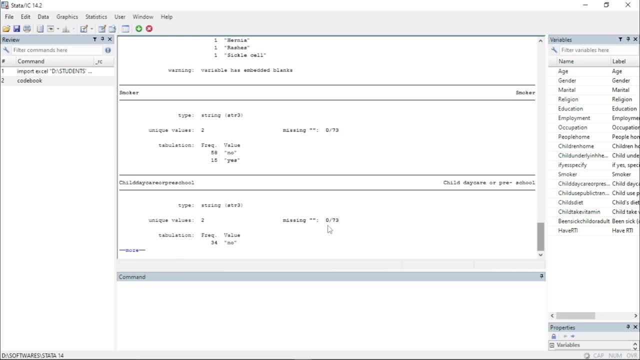 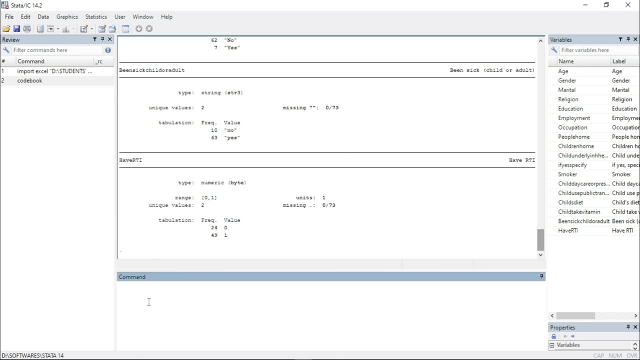 you can do codebook or you can be able to see other values or not in that, in that data, in that you know also, you can be able to see some of that information. now, having done that, you can do by the br browse to go and visualize how your data is. 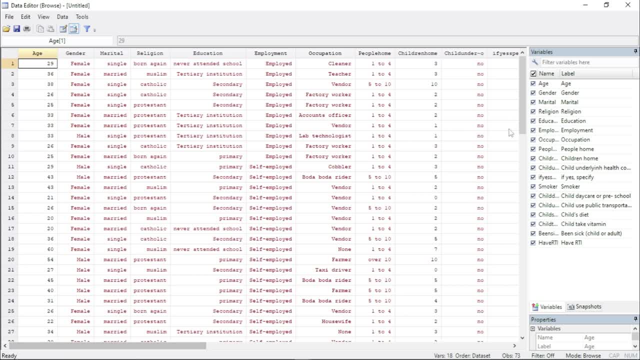 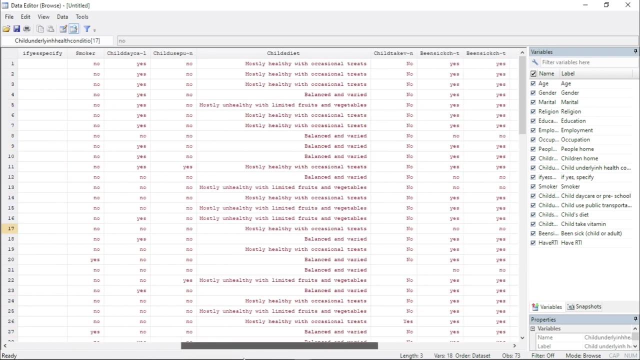 looking, if you do br- i always do br- if i go and see browse, i can see that. okay, every data set is here available. if you see black everywhere, that data set is black. that is a numerical data integer. uh, black. okay, so the the data set is black. 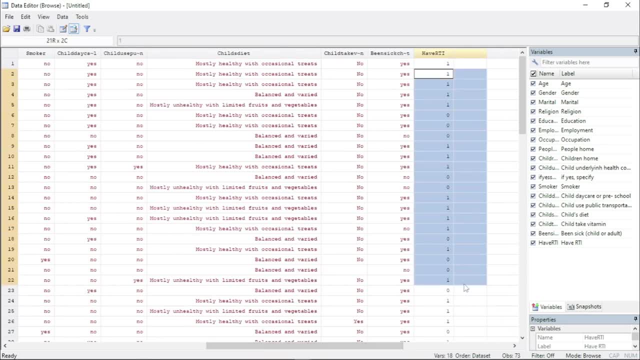 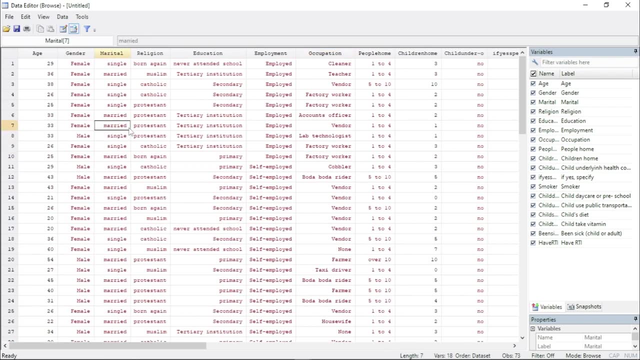 the the software has recorded it as numerical, black numerical, if you see red, those are strings. the the software has recorded as a string variable. now what you need to notice that, whereas you can work with some strings under starter, you can work with these strings. you can do things like tabulation that we're going to do. some other analysis: cannot, cannot, cannot, like. 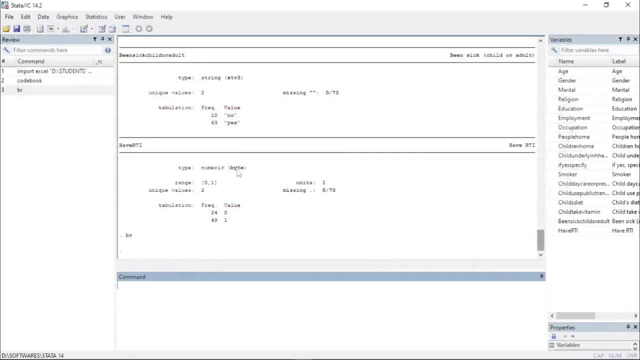 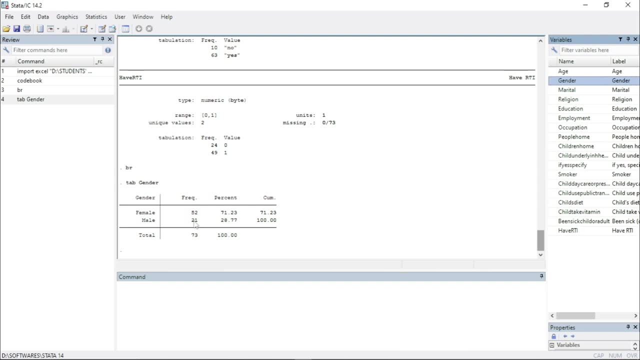 accept if you're having string, string data. we will see. let me just give a simple example. you can do a test to, let's say, gender and you can get an output like the frequency for the males, females and their percentage. that could work right, that could really work. um, but um, if, if you do um, let's, let's. let's say: 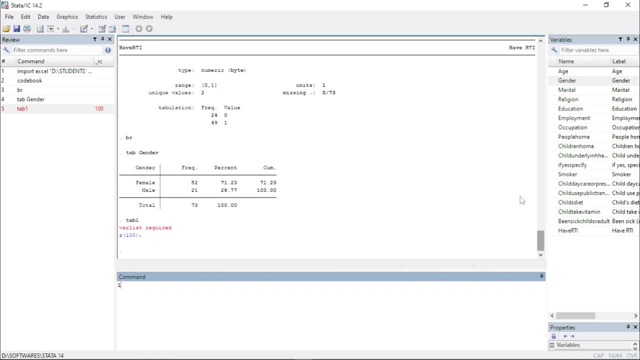 you want to do log uh, logistics, logistic, the dependent variable having rti, that is, a respiratory tract infection. then you want to to do an integration with the gender. you can see the error here. it is a string variables, so it may not be used as a factor variable, so you will not be able to do a logistic regression. 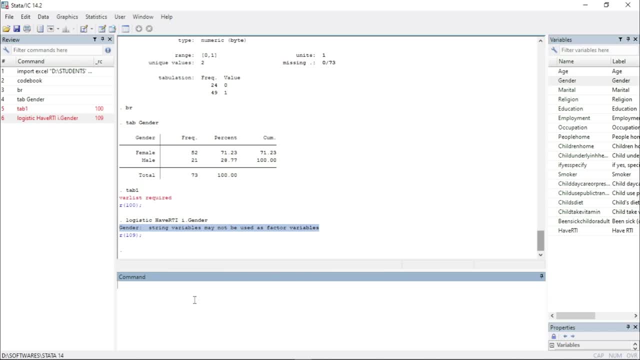 analysis because of the string. therefore, you will need to convert the strings into numericals. it is called encoding. so as soon as i import and i do codebook, the first thing i generally tend to do is to do encoding. i look for every strings, then i convert it into numericals. 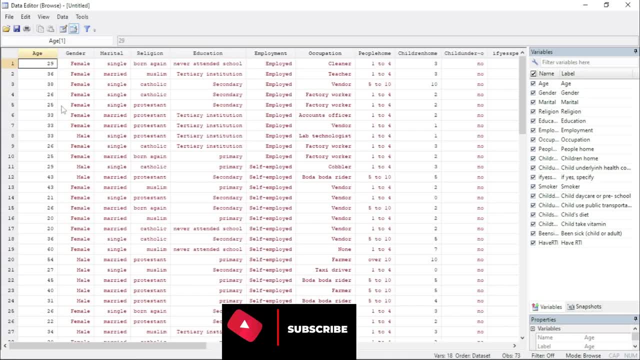 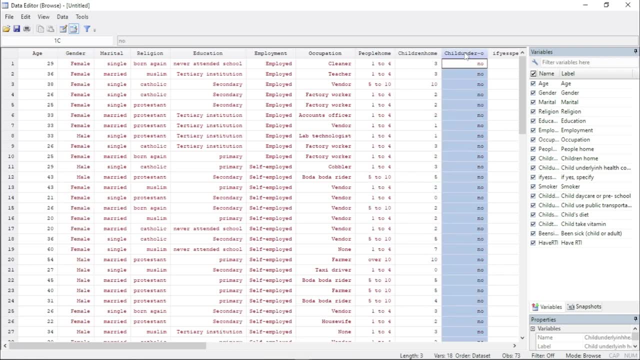 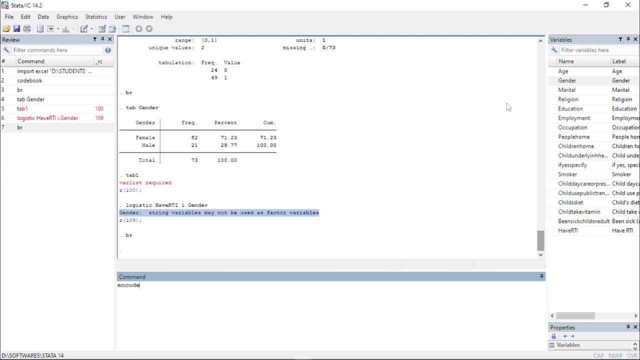 now from my data set. age is already okay numerical, so i don't need to. so i need to begin converting from gender up to people home. then i again leave: how many children are there at home? then i progress onwards. so let us encode. so encoding is a is a command in starter which is: 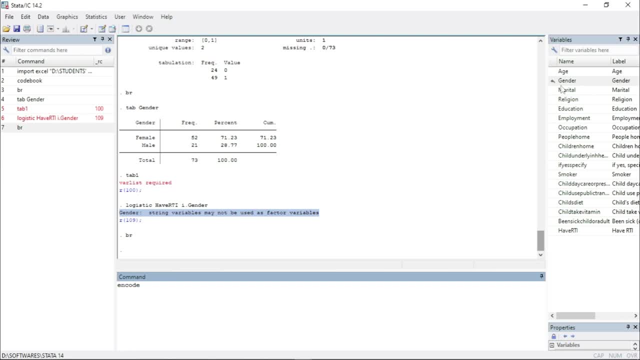 helps to convert string variables into numericals. so i do encode. i choose gender comma generate because you, you, you are, you're converting string into numerical. you need to generate a fresh variable, a fresh column, a fresh data, something like that. so i'll generate now, this time i'm generating a new column which has numerical data set of gender, so i'm going to then 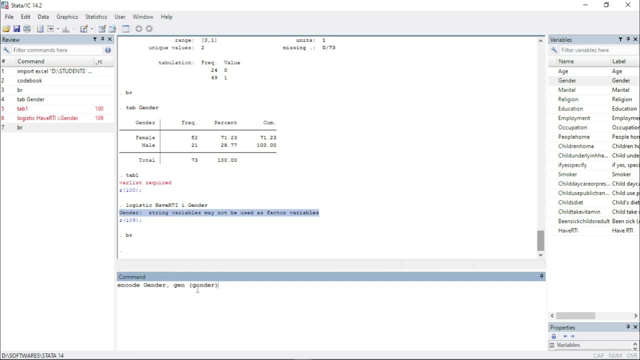 put here gender, it cannot go with the same name. if I put capital G, it will not accept because the name has we started different, not if I click enter, it has recorded. if you come on the right hand side I can see that it has created a new variable with the name gender and if you 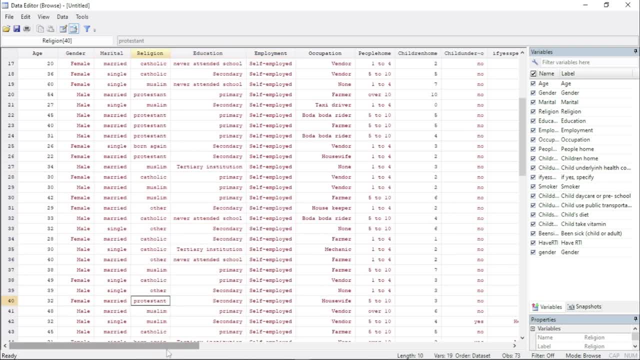 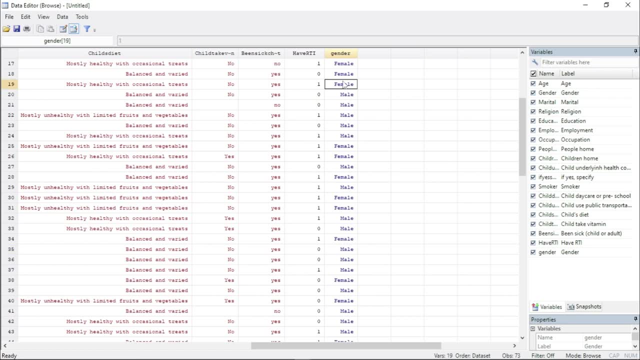 browse BR, you can go and check. and now it is in blue color. now blue color is in stutter. those are numeric. there's a numerical data which has string name, sort of like that. it has character names behind the scene. it is a numerical, but what you're seeing it is a name for all those numerical data set. so it makes it. 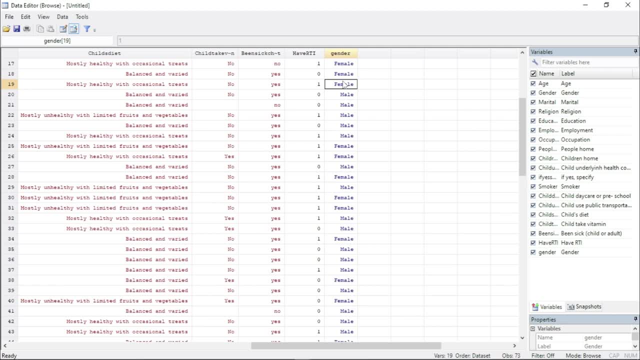 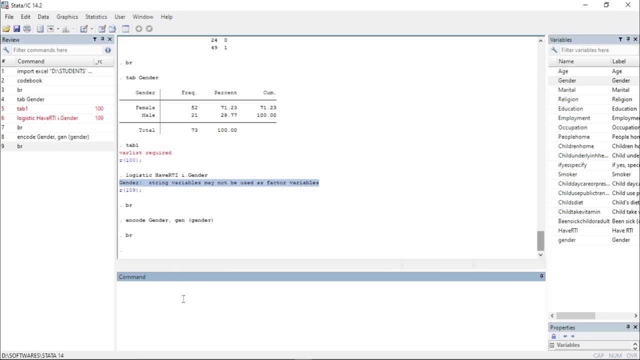 in blue. it means that those characters have a numerical attachment value assigned to them. so I need all my ready- should be bluish there, I'll be sure. so next let me encode the next encode: marital status. so this is going to take long. I'm going to rush through the video so that we finish encoding all the numerical. so 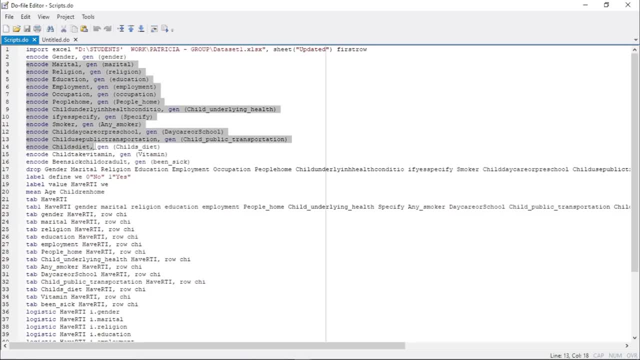 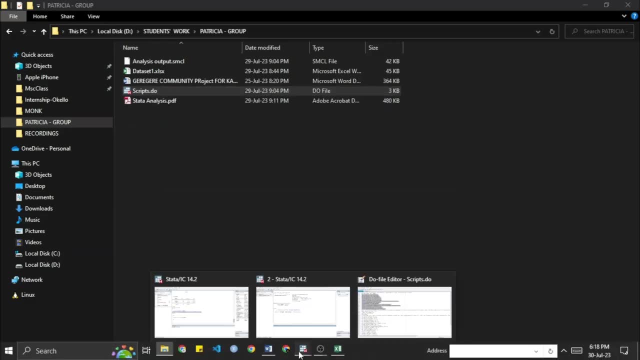 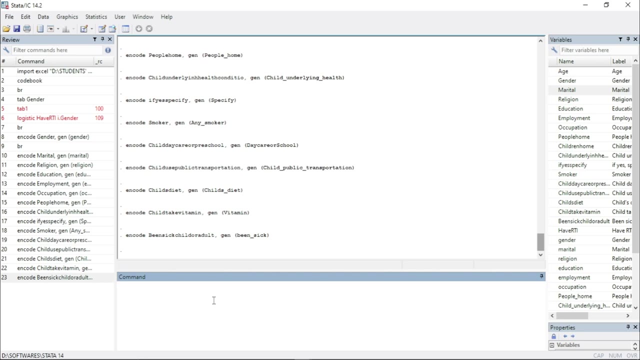 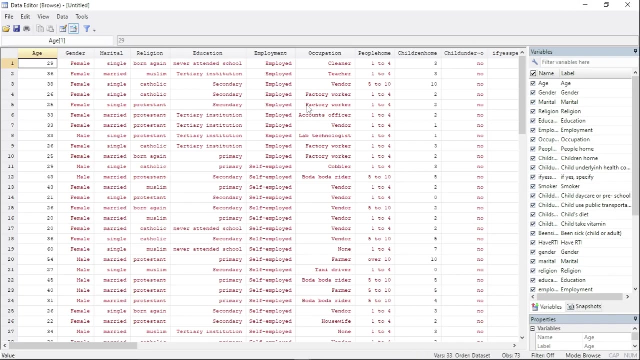 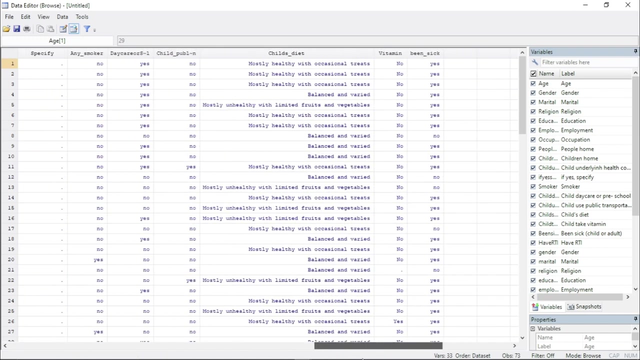 let me finish it up, okay. so I'm now done performing you that and encoding. so if I browse, I can now see that on top of this reddish one, if I go in the right hand side up, all these bluish kind of data set. so those 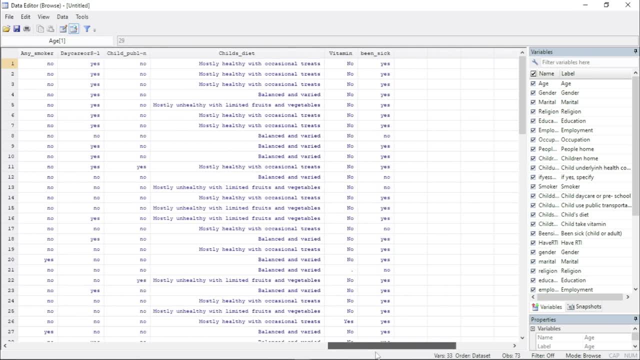 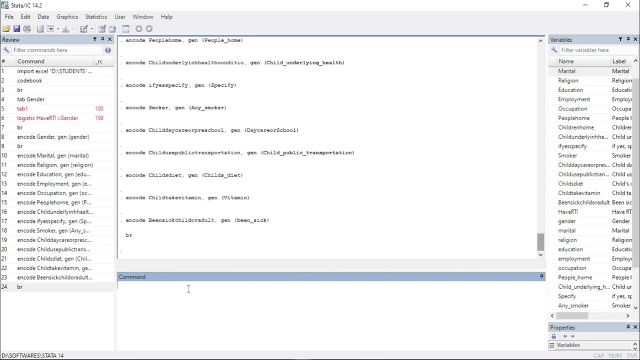 are the ones that I'm done encoding them. why should I encode them? it is because I want to use it, to then use it in further analysis. now I I therefore need to drop everyone that is string in here because it's not important. so I drop all the ones that are string because the cop is already created. so 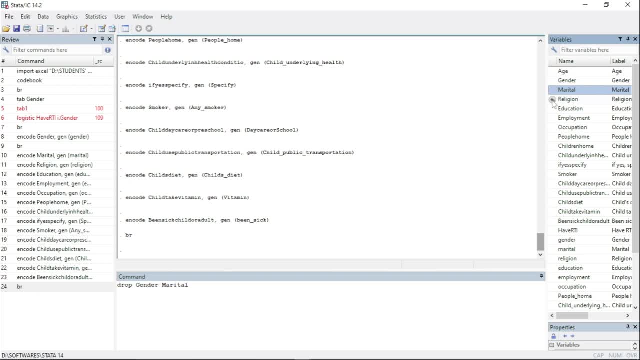 I'll drop gender, that strings matter, status, religion, education, and promise that occupation. people at home- those were numerical, so I will not. children home, okay, okay, okay. and then occupation: okay, I don't need that one. okay, that one is already dropped, so let's it remain. shall online condition if 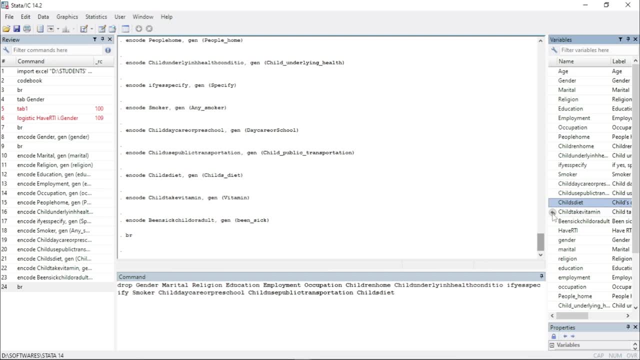 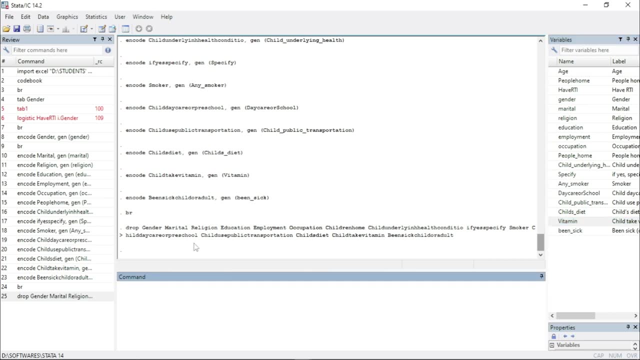 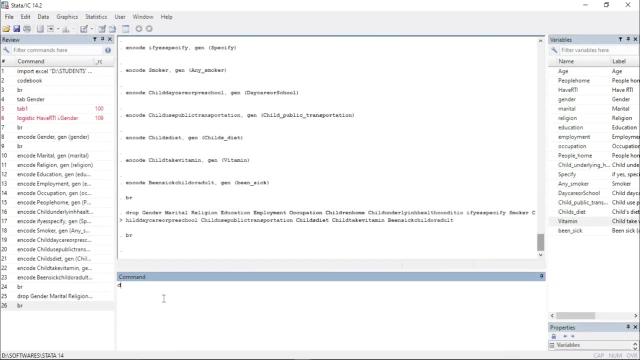 you specify smoker shall under pressure. so I remove all these variables and I stop. I don't remove half HRT. if I click enter, it has removed all those variables. if I browse, is the end of miss. okay, I've missed people at home. it's let me drop. 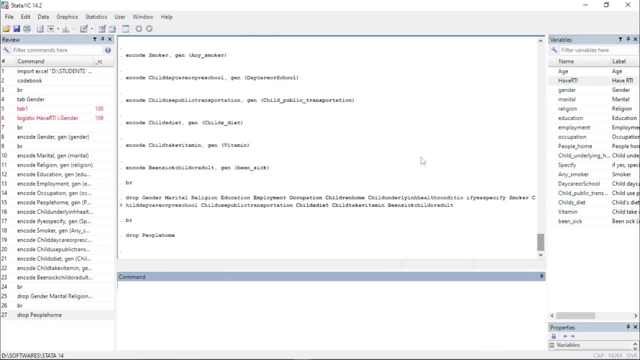 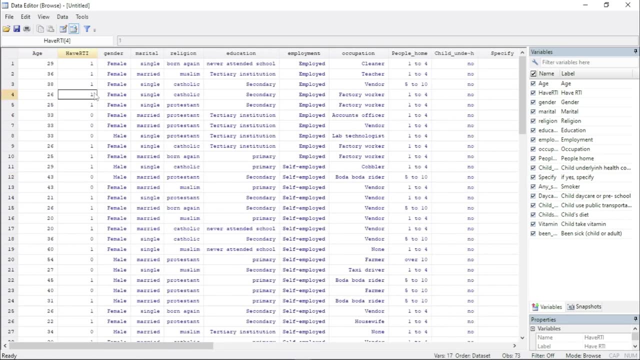 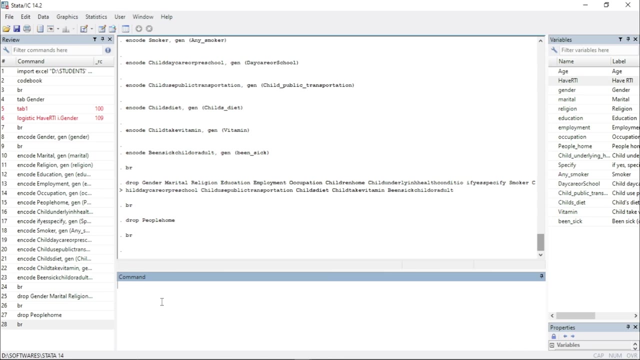 that one. okay, let me also drop that one. so when I browse, I can now see that I have only bluish and then the blacks, which are numerical. that is it now. having done that, I now begin doing descriptive statistics. so they let us perform descriptive statistics on this data. 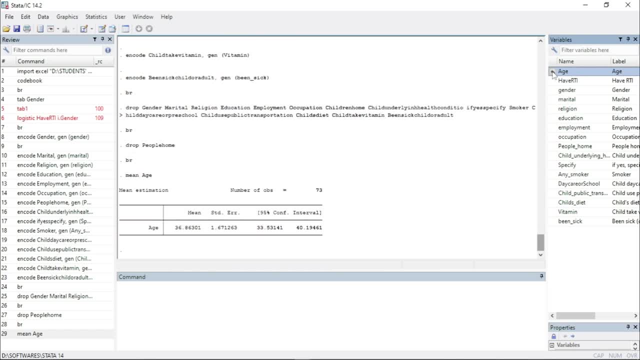 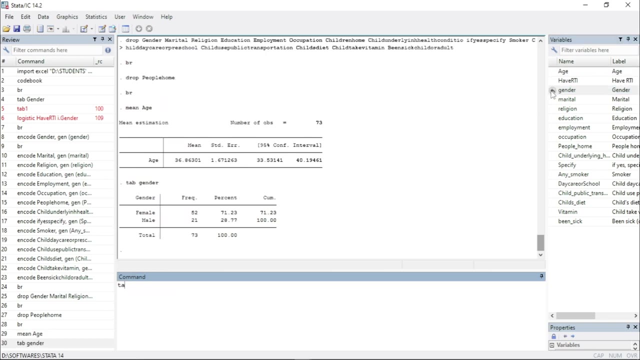 generally want to get harm. the mean age of the people that was 36.86. standard error is 1.6. that is okay. you report a new data set. you can then do tabulate gender, tablet gender. that is okay. it will give you that frequency and percentage which. 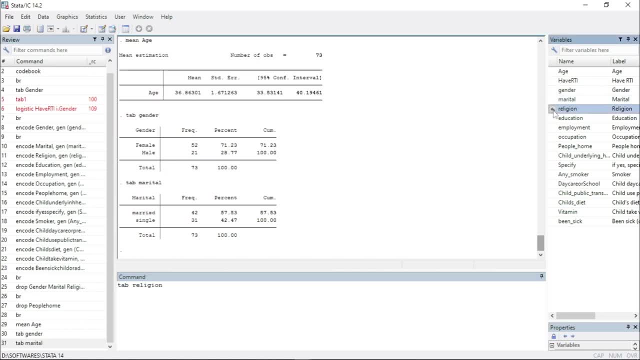 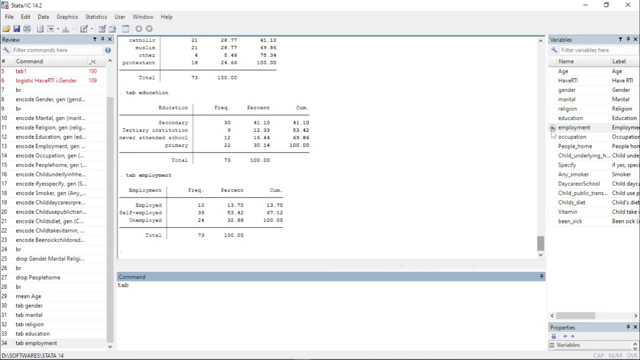 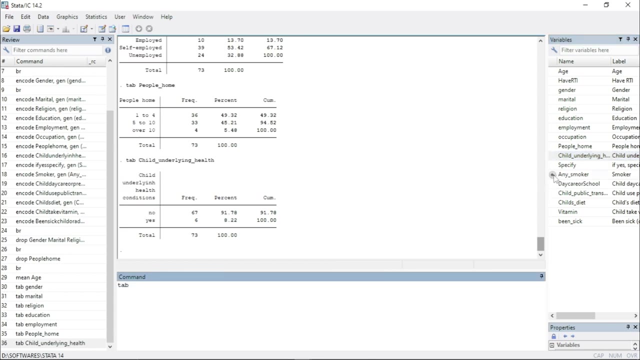 you need to report again a tablet, micro status. you'll be having another set tabulate. so you tablet all these are the categorical variables, so that you're able to have its statistics available. so I tablet shall, with underlying condition: you keep tabulating. so what it does, it will give for you the frequency of the 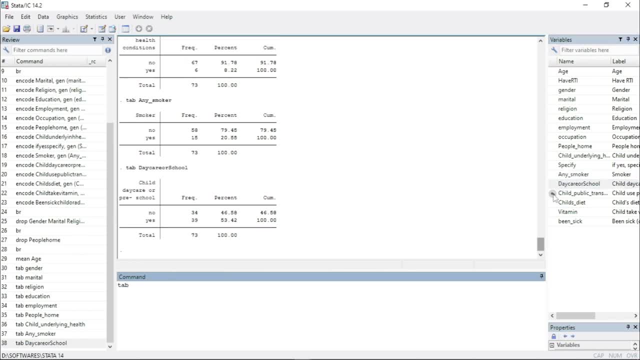 responses and its percentage, or what you call a proportion. I do that child's federal vitamin as a child ever been sick. yes, then I can also know tablet. my dependent variable is the child having respiratory tract infection, depending on what you study is. so you can then choose that and then you can see that. okay, that no 0 means no, so 24. 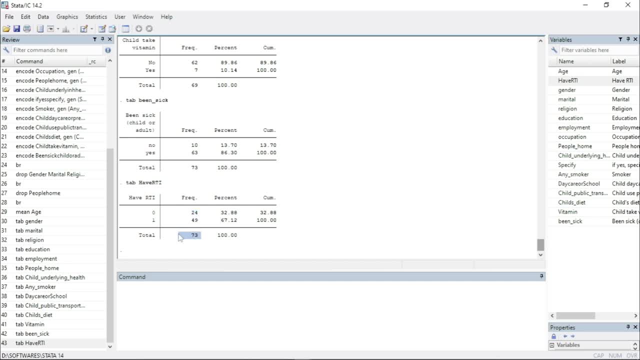 of the children are 24. four out of seventy three of the children didn't have respiratory tract infection, and then 49 added. and these are the percentages now, whereas we could proceed from here, uh, this dependent variable, again recorded as zero and ones, and sometimes, if you run the analysis, it 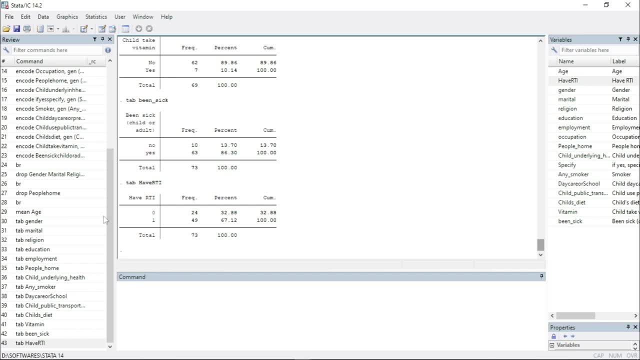 is really hard to interpret. why can't you name this zero and one? you, you give it a name so that you have, uh, yes, no, but yes, no in terms of, again, numerical data. so how do i convert zero and ones here to have yes and no? okay now. 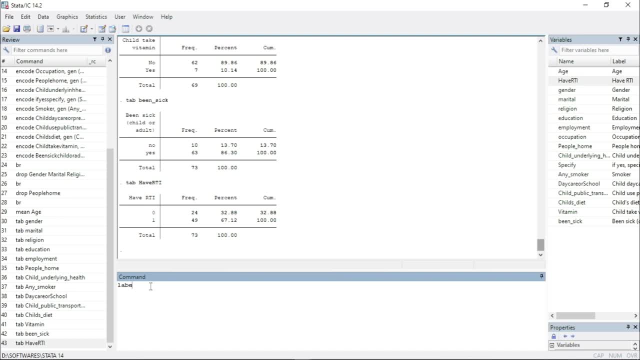 that is called labeling value, label value. so there's what you call label define, label define, you need to label define. you tell them that i want to label define. you create a label name, so i want to label find. let's say uh, ds, that you give it. you can do anything: one, two, three, four, d as any character. 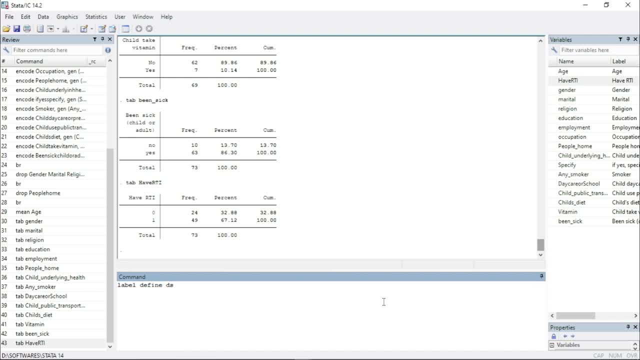 you're just giving it a title of a level definition, so i want, everywhere you see zero, let it be no or not infected, or maybe healthy it. it depends on your choice. let me call it not infected space. how about one? if you see one, make it infected or sick, something like that. that is my label definition. 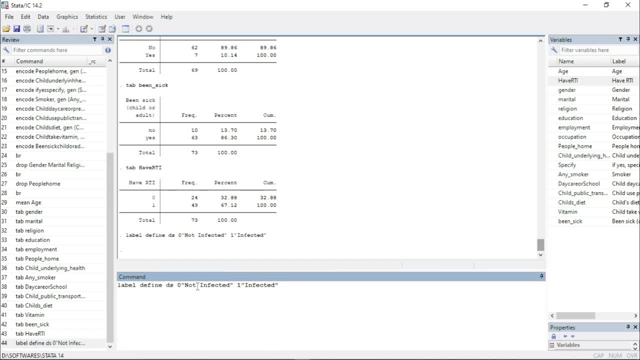 press enter. you need to put it in quotes, because now you're more like giving it like a character. so, whether zero give it this character, so those characters need to put it in quotes. that is how. so we have defined ds now. now we need to apply this ds into our dependent variable, which is: 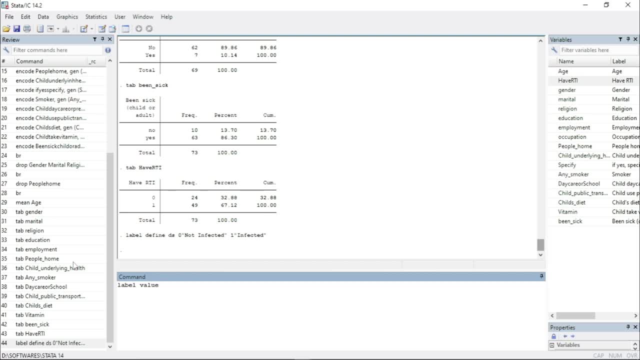 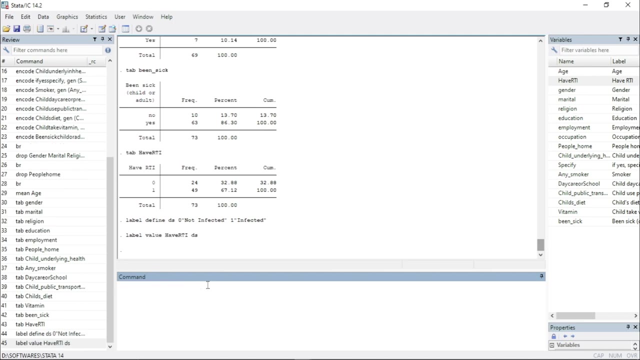 having rt. therefore, that is called label value. so we want to. we want to label the value under dt and we are going to label it using the key which is phone, under da. so you do label value what you want to change and then the key press enter. it has labeled. if you want to prove it out, 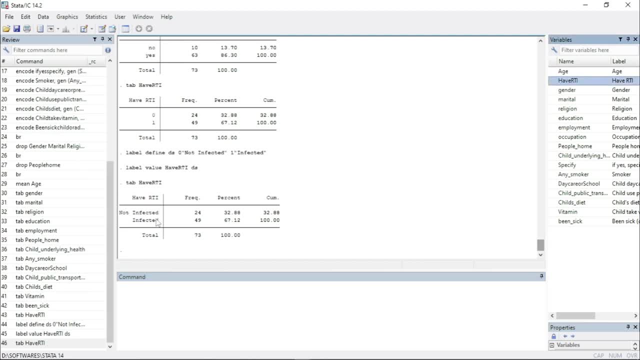 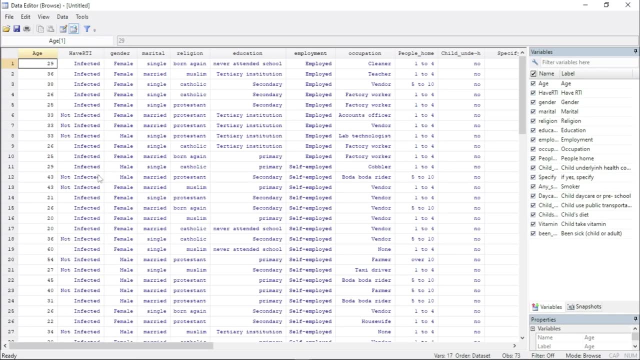 you can do: tabulate, have rti. you can now see it has changed all the zeros. it is now not infected. all the ones are infected. even when you browse br, you can even see a new data set. it's no longer 0 and one zero and one zero and one. it has converted it into now a character based. 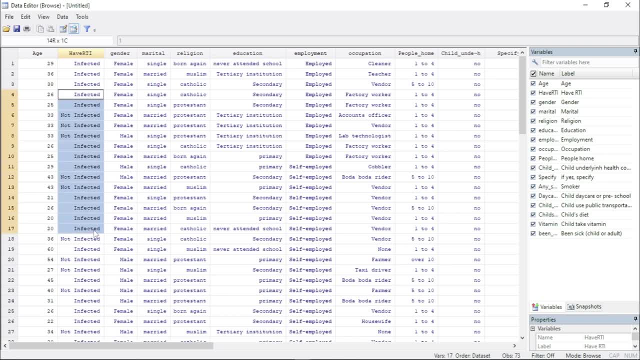 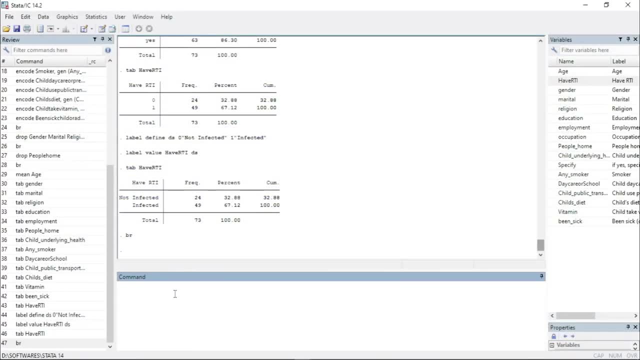 but it is blue in color telling you that, behind the scene, all these characters have a numerical attachment value attached on them. good now, having done that descriptive statistics, now i go ahead and begin doing a bivariate analysis. let me begin with architis. remember, the objectives are: 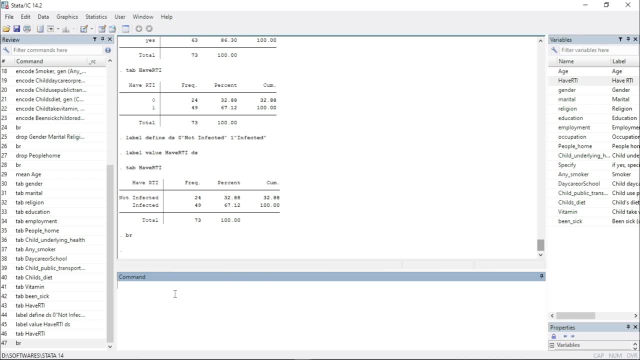 to determine the risk factors associated with somebody having respiratory tract infection. so all these other variables here are contributing factors, they are risk factors, but how can you then assess whether those risk factors are significant or not? so, basically, let me begin with a chi chi test, which will be a test to show me whether the distribution of my value of 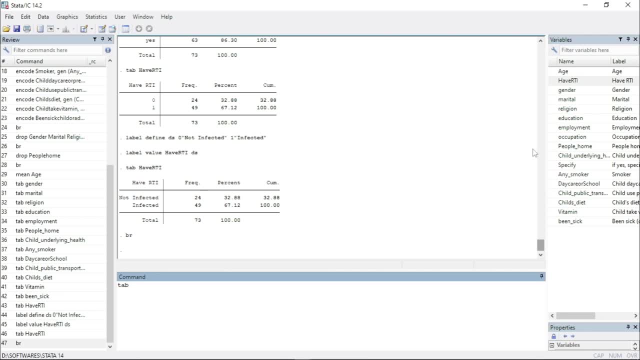 interest, that is, having respiratory tract infection. is it normally distributed like? is it distributed uniformly, or it is skewed, like some people are having more or not like? is it distributed? is it of a significant importance? are there? is it? yeah, is there something we have to worry about? is there a group? is there a factor? 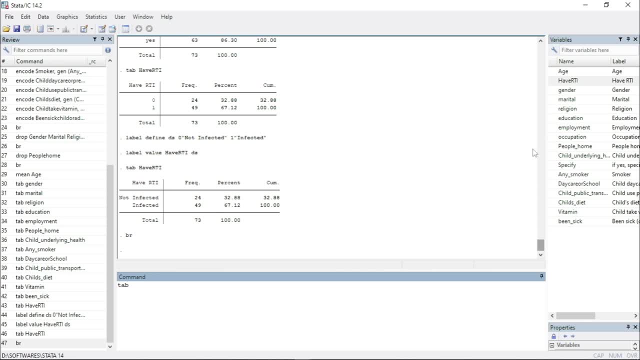 which is contributing most of some, something it's more like a distribution, frequency distribution. that's what chi test does. it doesn't offer you that, so that real direction, but it gives you an insight that this factor and this factor may be significant. so some institutions want you to do, some other institution doesn't want you. 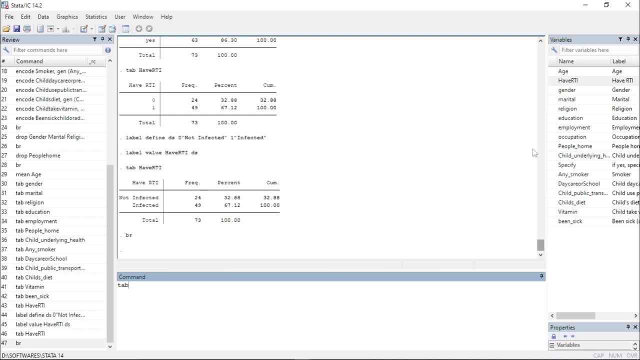 to do so. this step depends on whether your supervisor wants you to do or not. so chi test is gotten from a two by two table. it's a two by two, literally table. so literally i can just do a tabulation of um, of, of gender, versus uh, so that so. 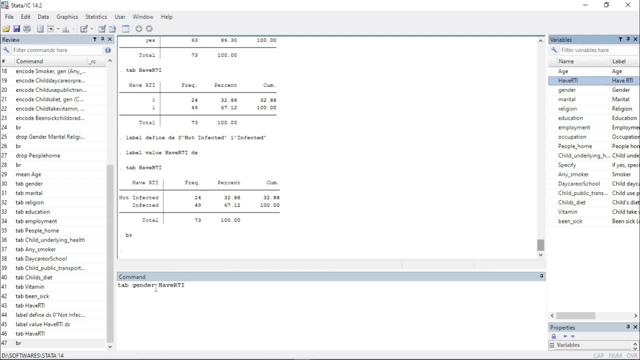 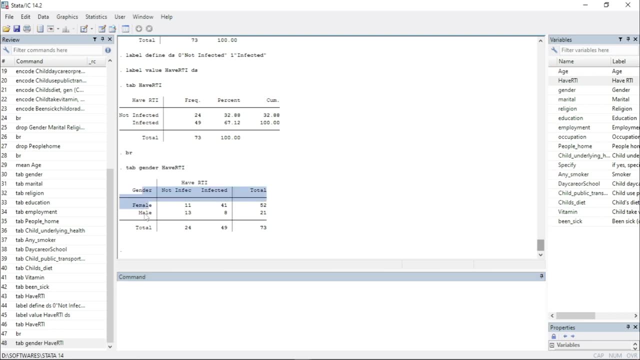 it is two by two. so i have the independent variable versus the dependent variable. if you only stop here, this would be a normal two by two where you'd only have a distribution of gender versus the your dependent variable. but this table you can, modify it, you can. you can say: i want. 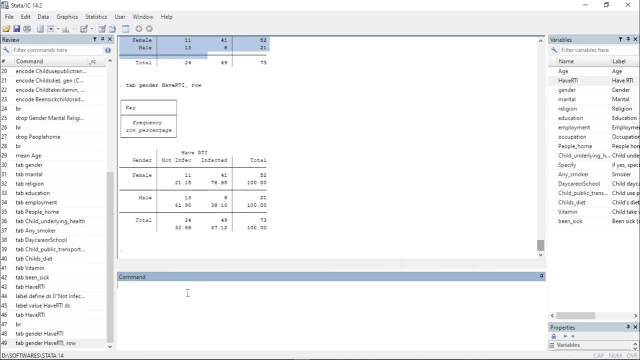 raw percentage. you just put comma, add row. those are what you call options. so on top will give you frequency. it also gives you the raw percentage that, okay, among is the females: 21 percent were not infected. 78 percent were infected. yeah, but also on the same one. 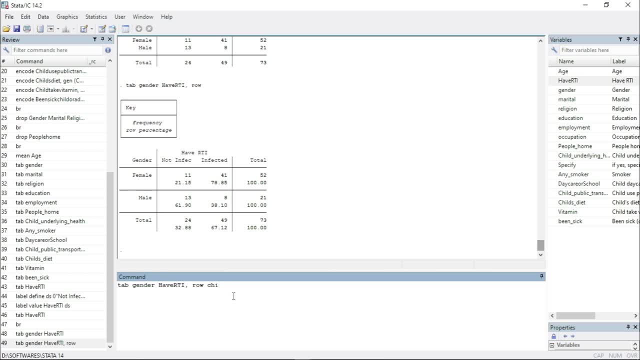 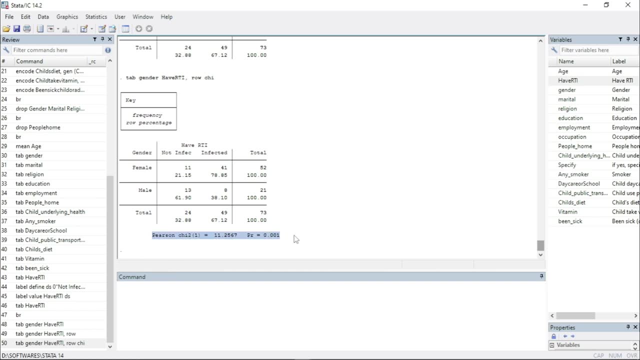 you can add. you can let it give you chi hi. so if you add chi, it will give you a chi value. right, it'll give you a chi value in here. so this would be an archive value to use. you can literally also do tabulation, independent, dependent, and then you you just put here: 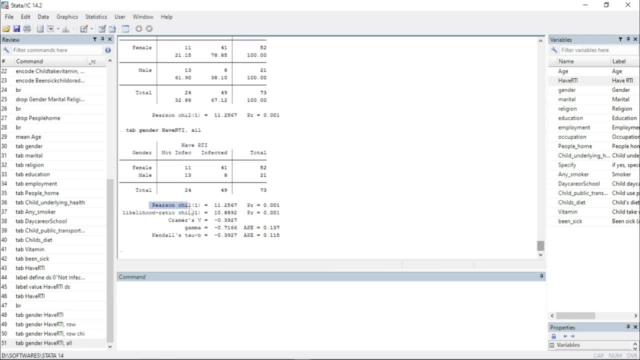 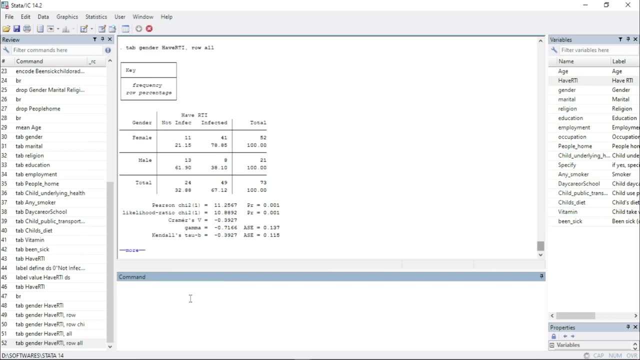 all. if you do all, it's going to give you these statistics here: pearson, likelihood, all these other statistics, or you can do tablet, gender, raw percentage, all, and then this one would be in terms of percentage and then you have the chi value. but from from from experience, most of the supervisor would only 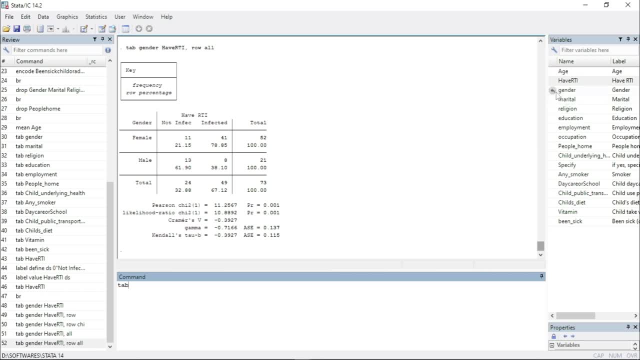 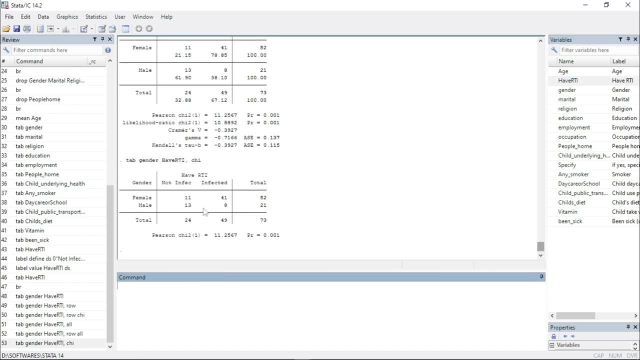 want you to report frequencies and then the chi values. i just do tabulate independent dependent comma chi, so you'd be able to have frequencies, that distribution and then pearson chi value and the p value. is this significant or not? so we can see this is significant, p value is. 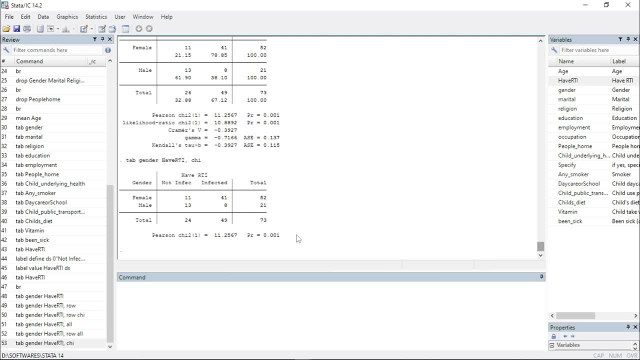 less than 0.05, by default starter will be doing analysis at 95 confidence interval. so significance will be concluded if you have probability less than 0.05. so that is a fair sign. but here we cannot tell that which of these is a contributing factor. 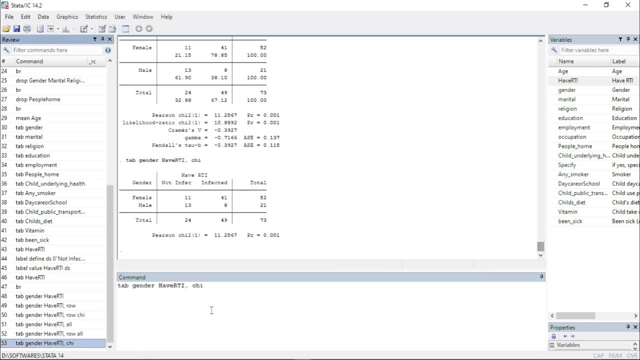 being male or being female, we can't tell in this case. but let's, let's, let's finish up those. so again, i'm going to fast, um, to, to, to, to fast forward the video, but literally all you're going to do is um, you, you run all these independent. 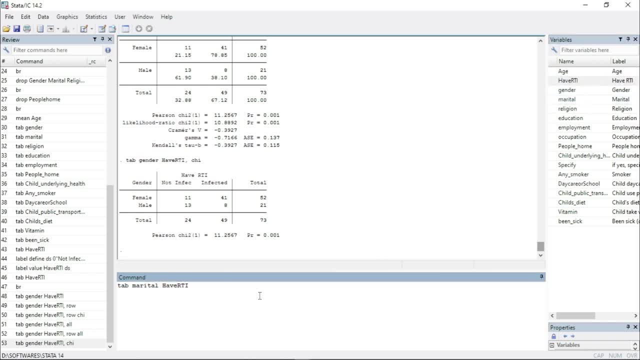 variables one by one and then you do archive value so you will be able to get all that chi input. you do tabulate. we are now going to religion- do having a respected track infection comma. then you add the value chi. it always will give you that that. 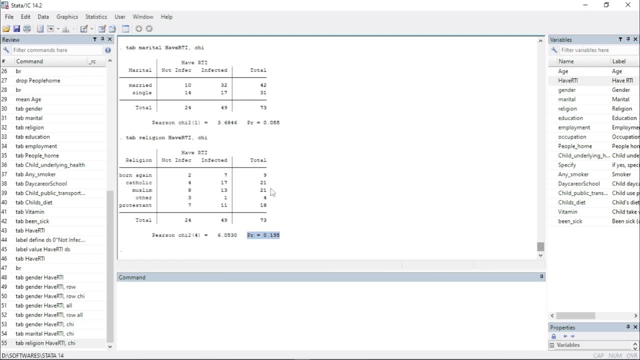 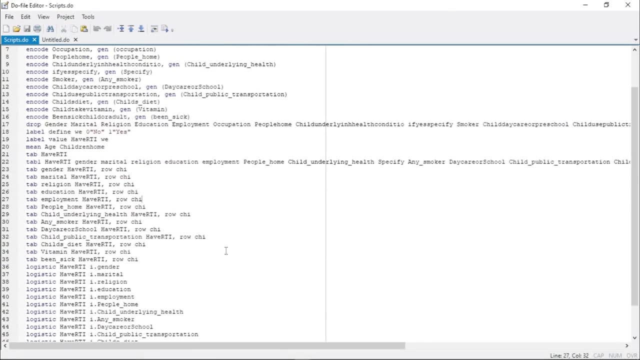 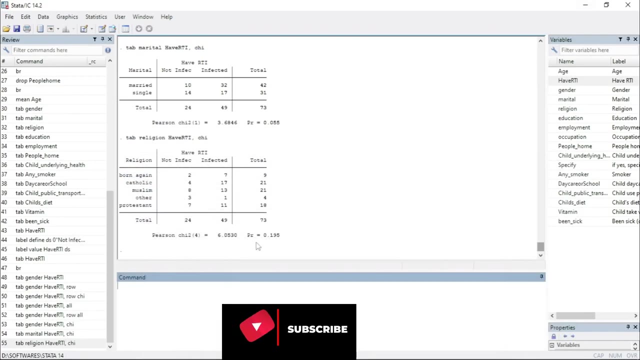 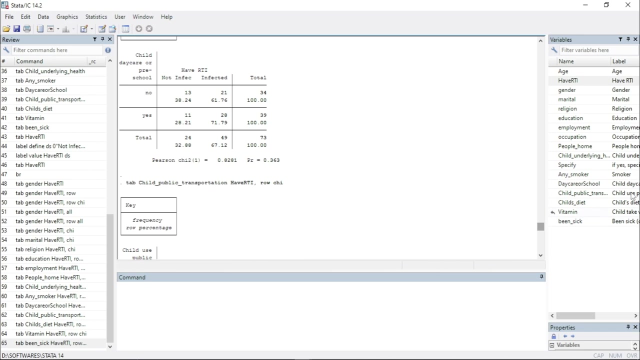 that information, then you'll be able to report that one accordingly, and it has respective p values in here. so, um, let me just run that first. i already created um a do file, okay. uh, let me just run that first. okay, so we're done with the the chi tests. it has gone through. 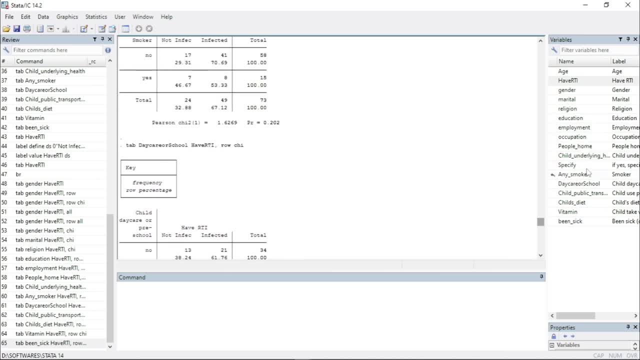 all these we have done through for each and every uh independent variables in here, versus our dependent, which is having rti, and we can see the p values here. uh, they are really more than 0.05. oh, this is. this is charles diet is also less than 0.05. so charles diet. 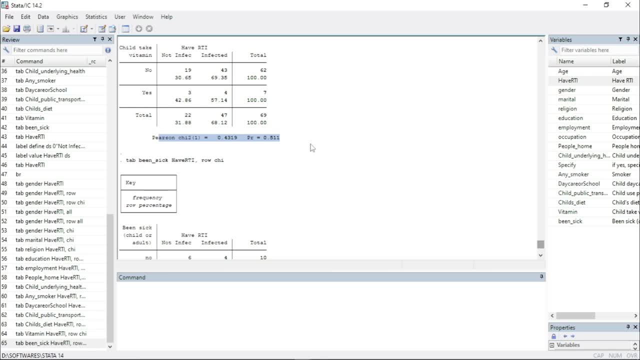 alongside gender. they're significant um having taken vitamins not significant associated. this is also significant because it lessens 0.05. so has your child ever been sick in some previous month? yeah, so that those kids are. significantly they're more likely to have respiratory tract infection, maybe because of their immune system has gone. 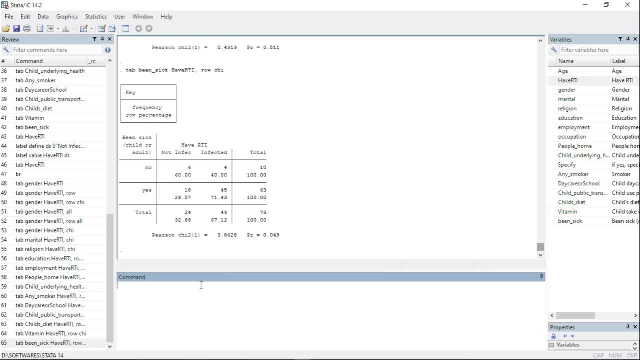 down one way or another. now we're done with this one. now we have to take it notch ahead and then we do some logistical regression. i get some odds ratio to logistic regression. i get some odds ratio to logistic regression. i get some odds ratio to look at which group had more likelihood of having the intersection compared to their. 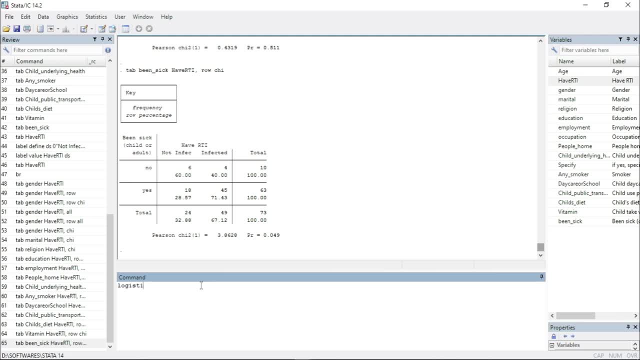 counterpart. so the command you would use here is: logistics- uh sorry, logistic. and then you would choose um, your dependent variable, and then there in the, and then the independent variable you want to regress with, and then, before that independent variable, you add the i dot, i dot, logistic. 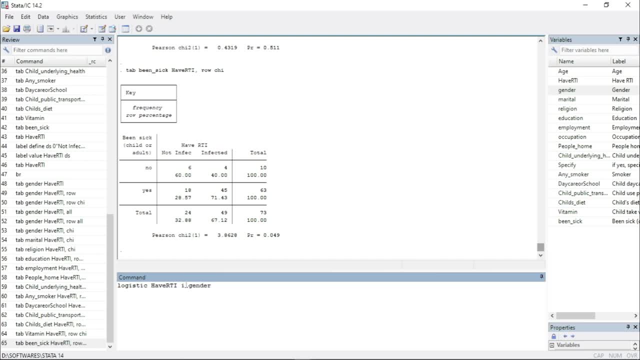 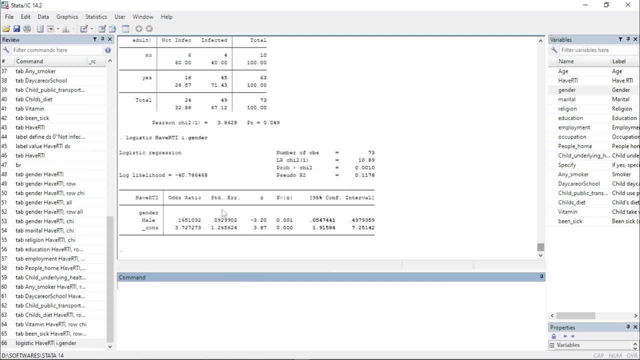 your dependent variable, your independent variable, then idea i dot to sign for like, like, like to tell you to do a logistic, a logistic regression, like on, on that, like something like that. and so if you run, uh, it's going to produce for you this output and it will give you this odd ratio, this odds ratio, which is very important. 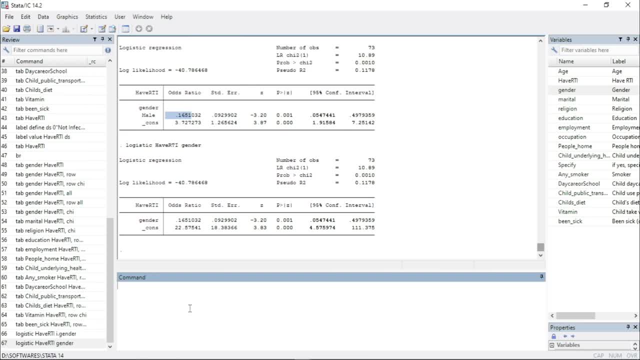 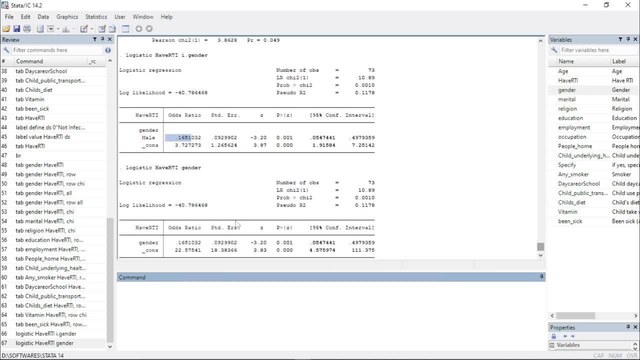 let's say you did not put this. i let's see, would it run? it still would be able to give you something. okay, but that would of course be a risk factor in there because if you look at, these values are a little bit different: the the down one, that is not important. the upper values, which are up here, is the most important. 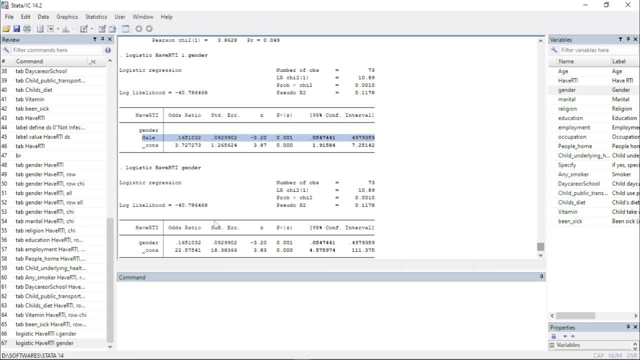 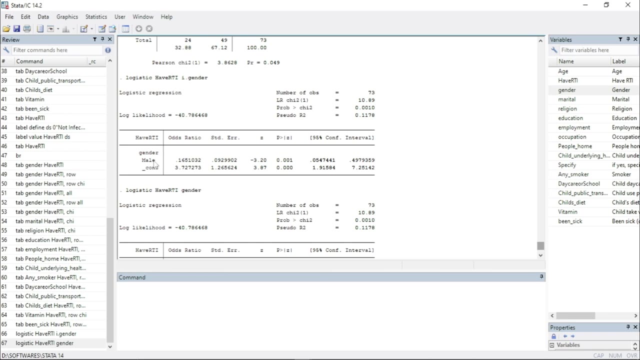 thing. but the challenge is that it does not give you a category. look at up here. we can see that female is hidden, but male is here. let us first interpret this up one first. this up one means that what if you're running a logistic regression, starter is going to pick. 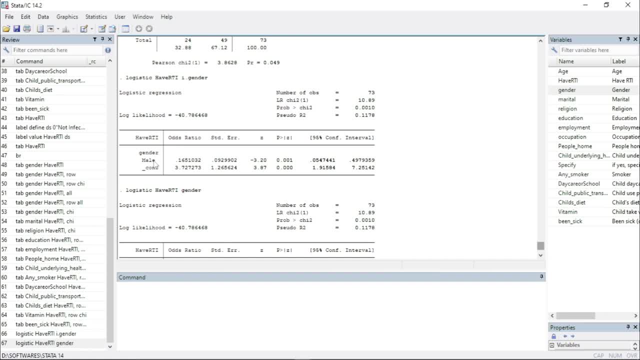 one of the response to act as a baseline for you to compare one against. here. we do conclude that male children are 0.165 times less likely. the standard is 1: 1.0. so by default, the value which is picked to be the reference is given odds ratio 1.. so by default, in this case, female is taking odds. 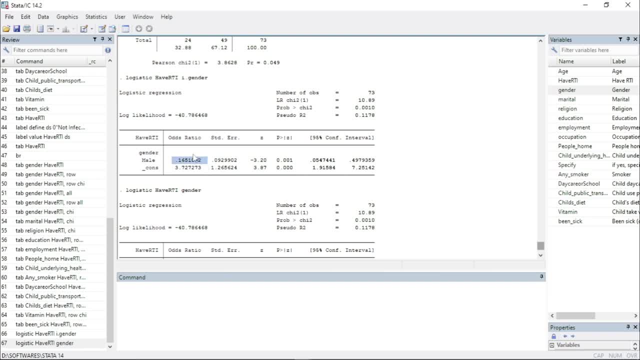 ratio 1, and now we are comparing male against the female, towards the likelihood of getting infected. so here we can conclude that male children are 0.165 times less likely to get respiratory tract infections compared to their counterparts who are female. and here is the probability. it was significant, so it is a significant um. 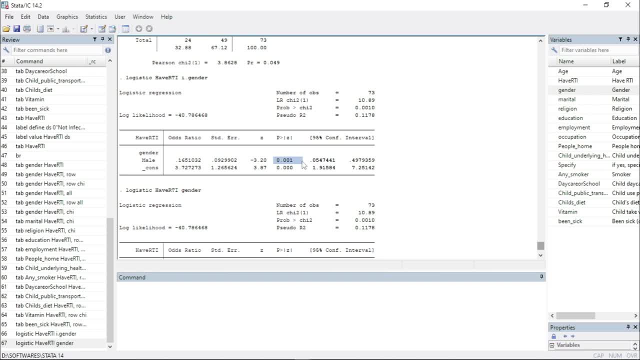 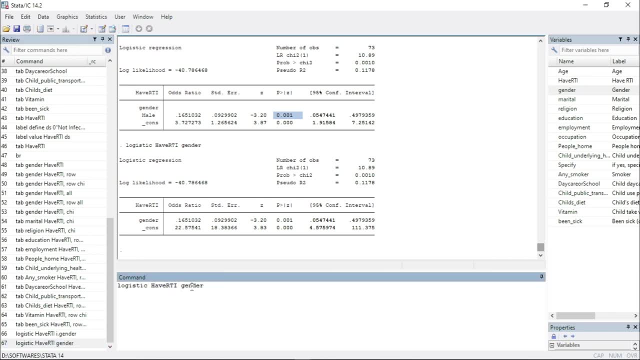 variable like gender is significantly associated with having respiratory tract infection. but if you run a command logistic and then you do not put i dot, look at what it does. it only gives a plain value. it does not separate for you. what are you comparing against? male or female? it is. 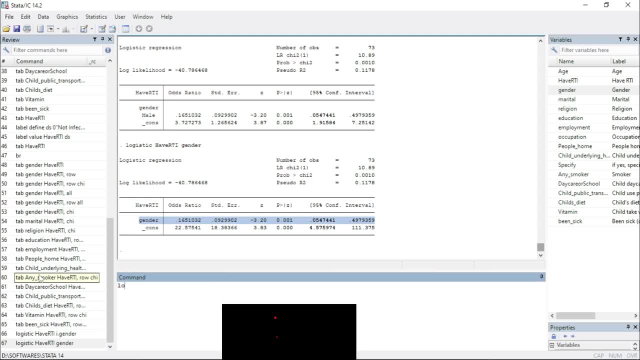 hard to tell. in that case, let us try something else. if i do logistic and then i i do, um, let me, let me get something with more than one category, let me do education and then, having respected, i mean, i need to begin a respiratory tract infection first. so i first begin with the 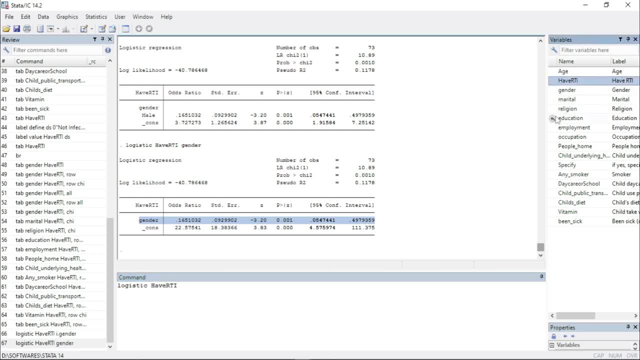 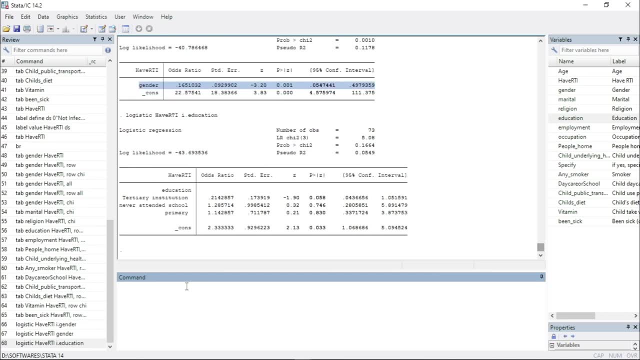 respiratory tract infection. that's the dependent. and then you do um, education. if i do add, i here, okay, it goes through, right, everything looks to be okay. but um, if i remove, so here i can easily see that okay, primary: never attended school. tertiary: there is no secondary, so secondary. 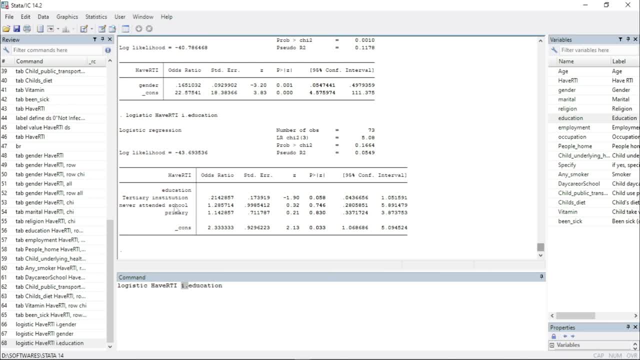 in that case is now the the the best thing we are. we are comparing against. so in this case i would say: people, uh, children with the parents who have reached tertiary institution are 0.21 times less likely to have respiratory tract infections compared to their to to to their counterparts. 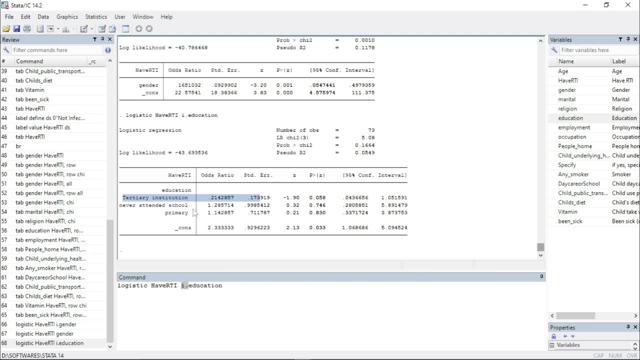 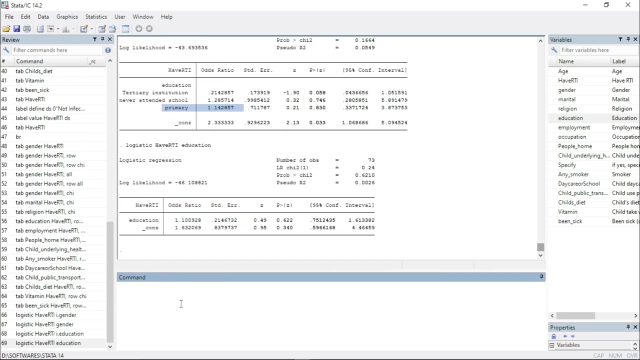 whose parents only have secondary level of education. children from parents who had primary level of education are 1.14 times more likely to have respected tract infections compared to their counterparts, uh, whose parents had secondary level of education. that that would be a conclusion. but let's say that command had run without an i. what would happen? look at what it does. it only gives you. 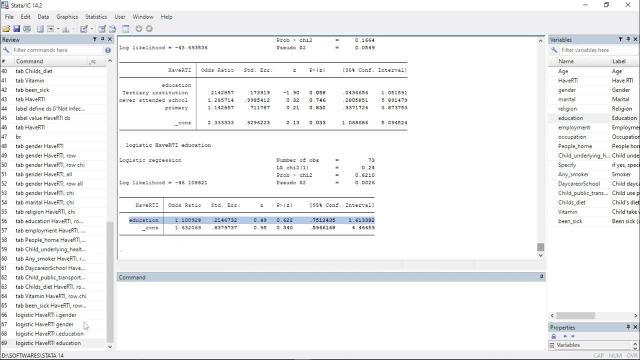 a uniform kind of value. in this case, you cannot draw conclusion based on this. so when you're going to run this analysis, make sure you have i somewhere there. there is also another version of running this analysis. i think it is legit, legit, legit. and then i put, uh, let's see. i hope it works out. i put my 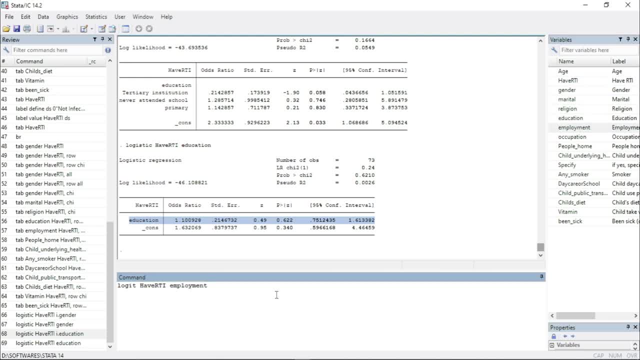 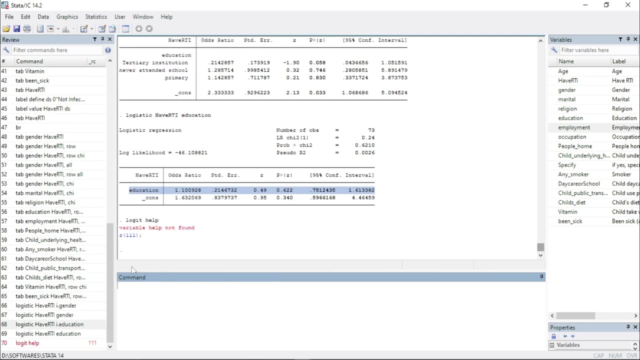 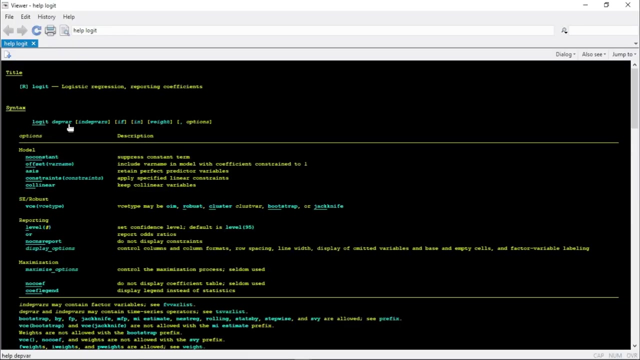 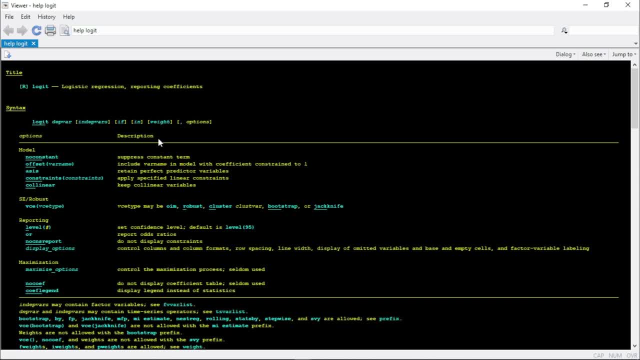 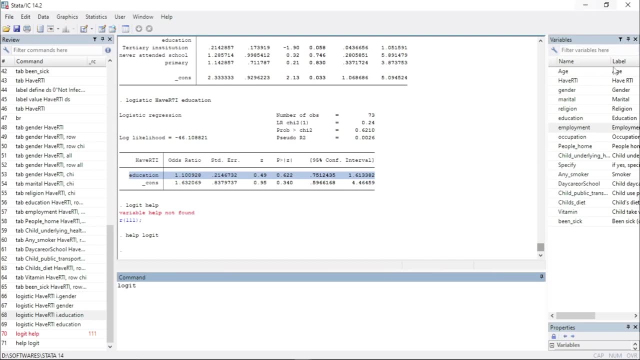 okay. and then you need to add independent variable, and then there are options. let me see the options in here. i want an option of regression, okay, so there is. or you need to add or to report odds ratio, because i need odds ratio, uh-huh, okay, so in that case i'll do logit. our dependent is having respected. 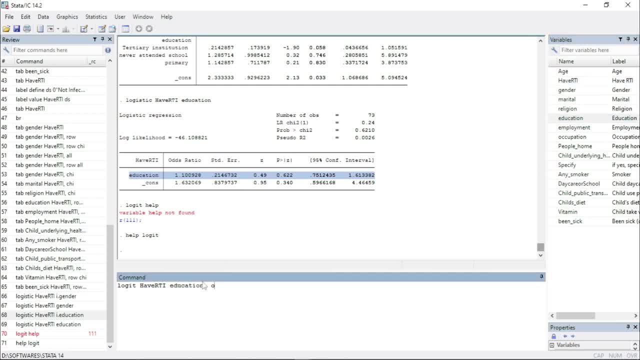 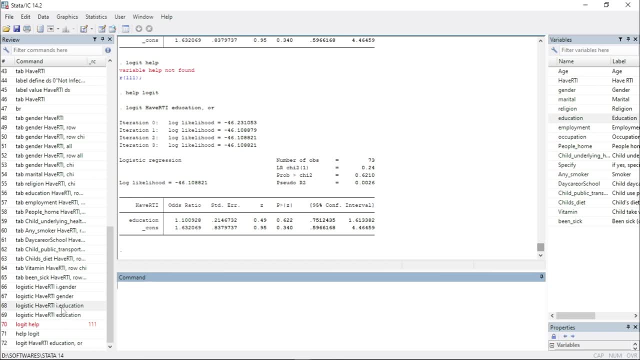 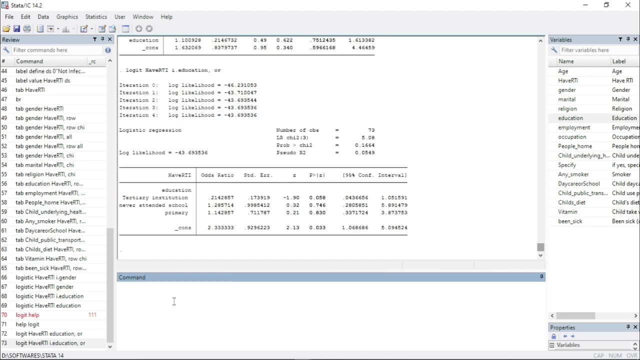 track and infection, let's say education, then your food comma or r, uh okay, it has still given a similar thing. so i think in in that regard there is, there's no hope and i know that with the, with the logit, still i may need to put i there, so you cannot run away from. 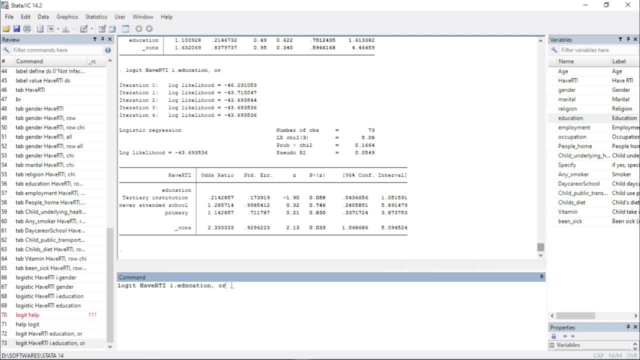 i. i think what is special with the logit is that if you use uh logit and you don't add this option or r, it does a report for your odds ratio. it reports coefficients instead of odds ratio. so the the option for dependence, then you have an i in before the independent remains. 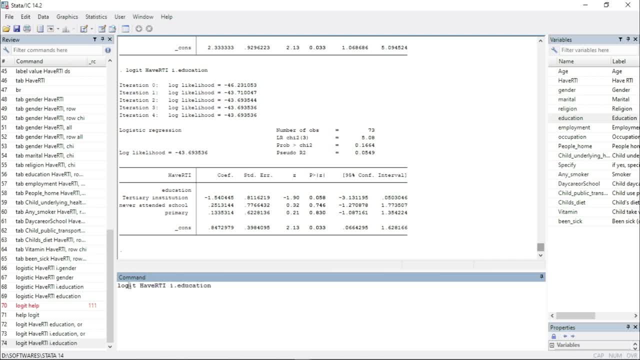 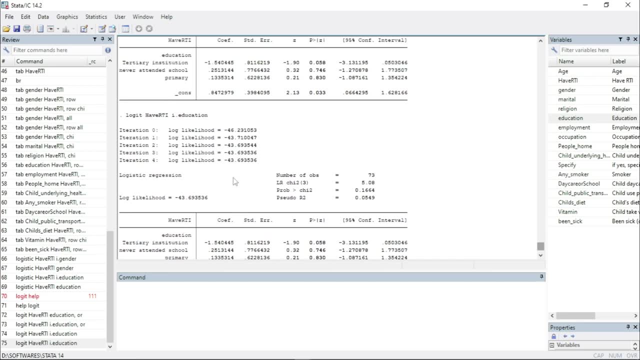 constant for both logit or logistic. but if you use logit and then you run logit only, you will not be able to have odd ratio. you'll have coefficients on there. but if you want odd ratio then you need to add comma or r and then it will report for you. 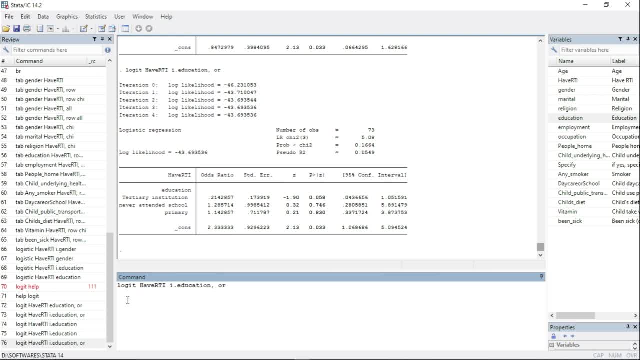 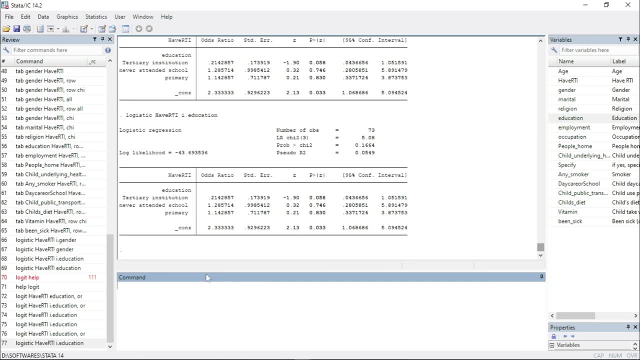 the odds ratio. but alternatively, you'd, rather than have here logistic and then you have dependent, independent, then you remove this or it will give you the same uh output. so that is another version in there. so that is what, what? what would be a drum logistic regression for all these uh, uh, dependent variables? 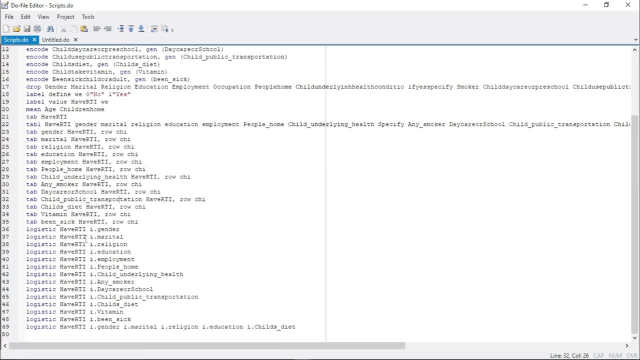 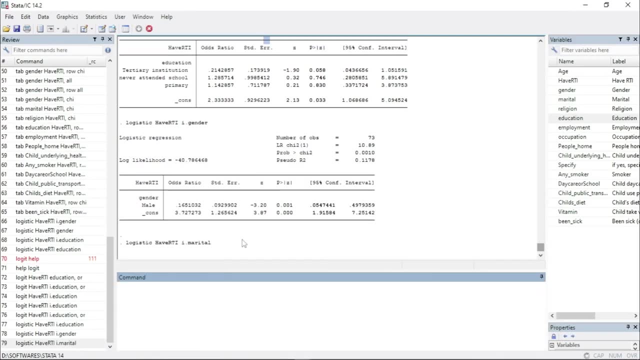 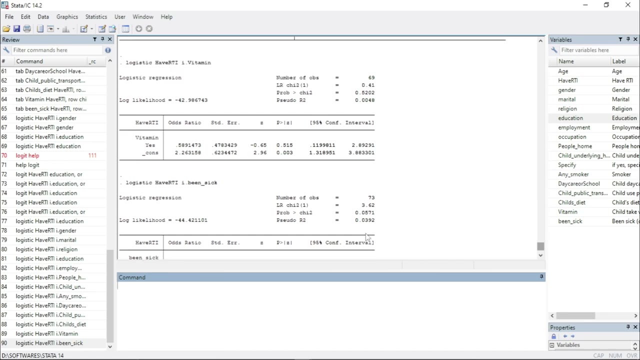 so let us fast forward. uh, on that. so logistic regression we are now. so you just do all those logistic regression one by one. of course, this one already performed one by one, one by one, so you'd be doing this one by one, one by one for all the variables. 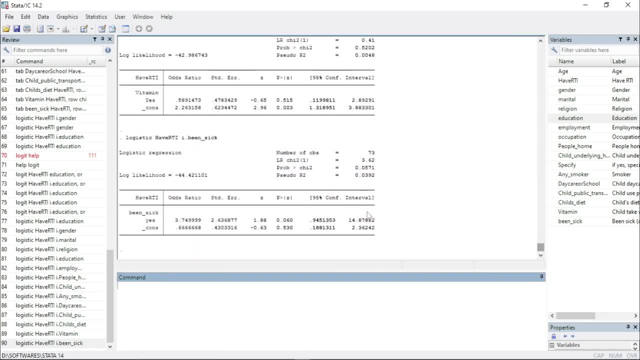 now. i will need to then do multivariate logistic regression to remove what you call the confounding factors. how? let me explain that, although we are saying gender is associated with the respiratory tract infections, apparent educational level is associated with it. so you realize that by the time you have that infection, it may be, you may be. 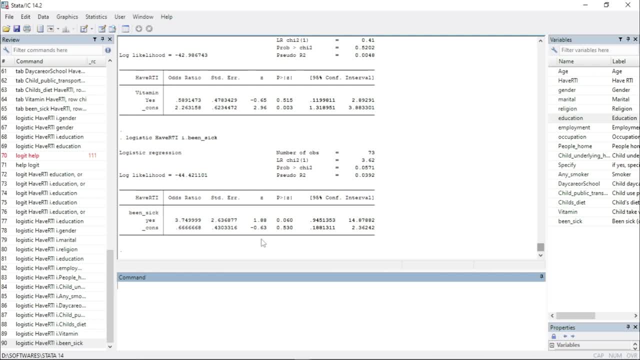 having multiple factors that may contributing, uh you, to having that infection. so all those factors are called the confounding factors. so we are saying that it is hard to draw conclusion that gender is really a significant factor or whether taking vitamin is a significant factor. therefore, you need to do what you call. 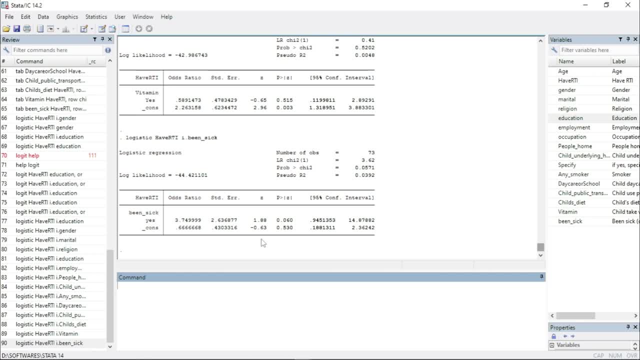 the multivariate logistic regression so that you're able to rule out every variable that may not be a true significance, a true significant. now there are rules to for doing multivariate, there are rules upon it, but uh, i'm not going to talk about in this lesson. but you're supposed to have, like 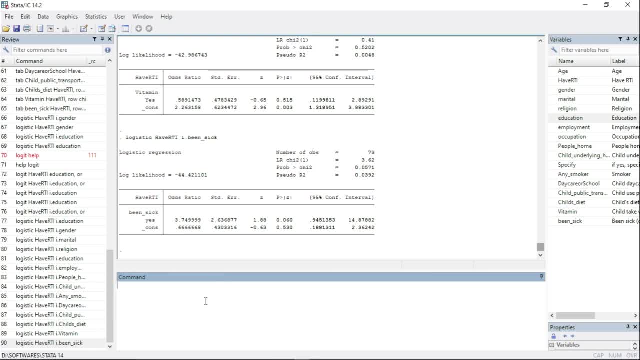 you only cut off from a certain p value. but in this case, let's, let's drop that off. let us say you need to run logistic uh for your uh dependent variable. again, it's all other variables, all other independent variables, everything from gender, micro status, religion, education, employment. 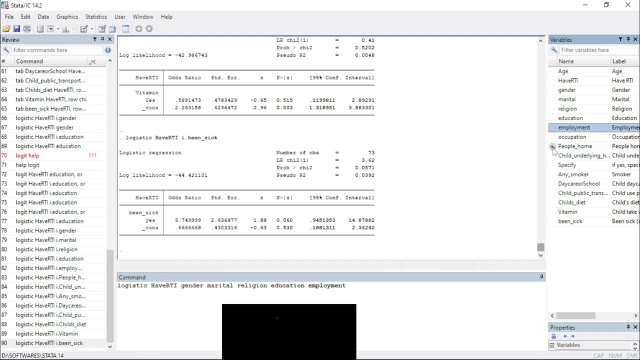 um, okay, um, how many people do you have at at home? is the child having online condition? uh, is there any smoker? is the child going to school? does the child use public transport? does the child have good diet? does the child take a vitamin? has the child been sick? i want to to do this. what could a multivariate now you? 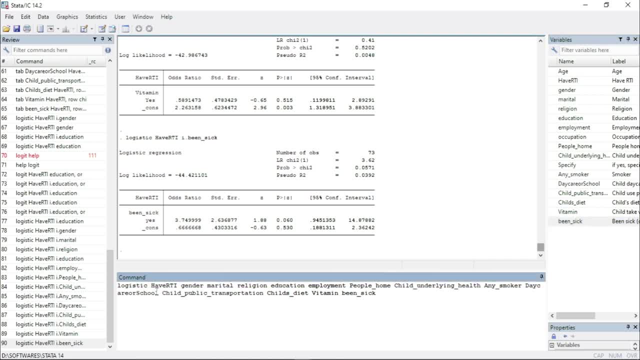 consider all the independent variables at the same time. in this regard, you then need to regress, so i'm going to be regressing. this again is so you need to be adding. i again. it's that, again it's that, so you'll be adding, so that you do you get odds ratio for all these. 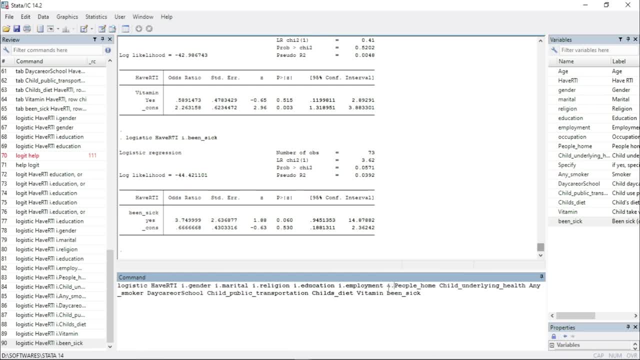 variables now. the difference is that the odds ratio from here it is called adjusted odds ratio. adjusted odds ratio: if you do a bivariate, you call it a crude odds ratio. this is adjusted now. this adjusted is much more preferred. it's much more um reliable now because you consider all the variables at the same time. 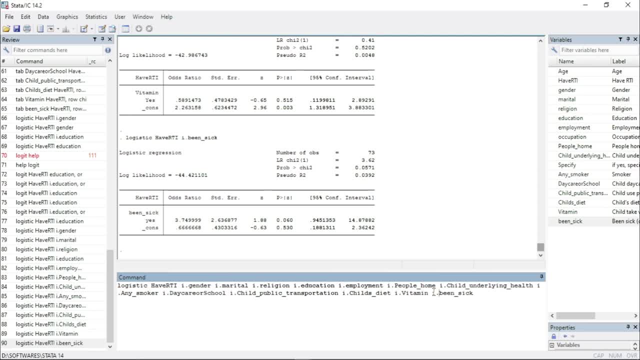 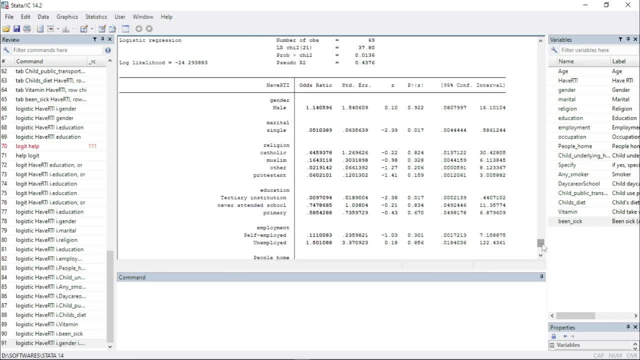 so any significance you get from here is now a true significance. now let's run that. so when you run it, it will give you an output in one table. so it has not compared everything at the same time, and it's it has still given you the, the odds ratio. 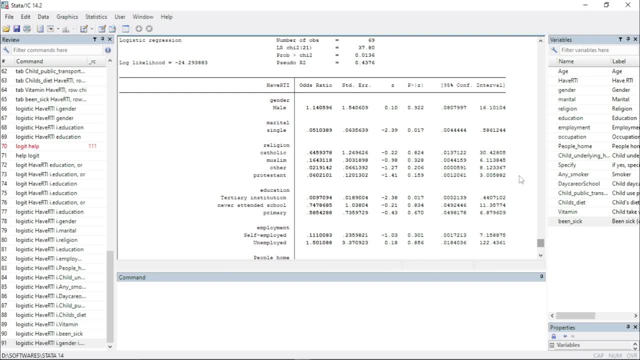 but in this case the values are now somewhat different. now let us confirm. remember when we did bivariate, we said that gender was significantly associated with the infection. now look at what's happening here. it's not in reality. it's not. if you go back to to a bivariate, let us run a bivariate again. we remind. 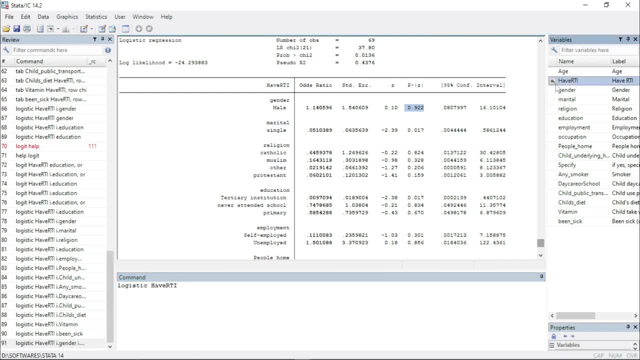 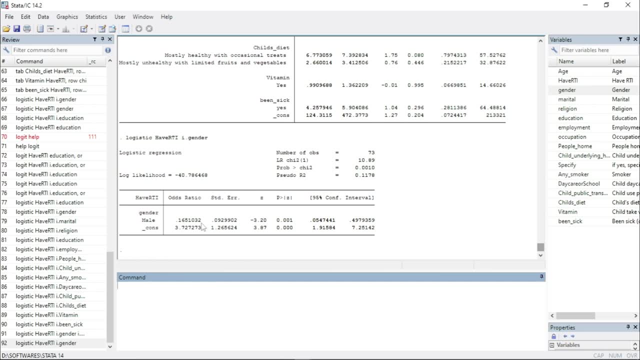 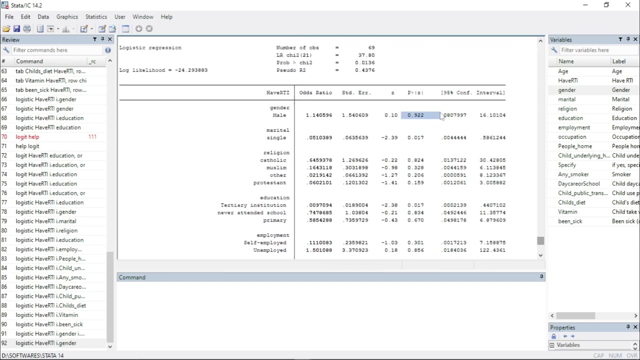 ourselves logistic. i want to run having tract infections. and gender, then i do. i add that now, if you look at here at the bivariate it is significant p value less than 0.05. but at multivariate p value is not so meaning gender in. in truth, gender is not a significant 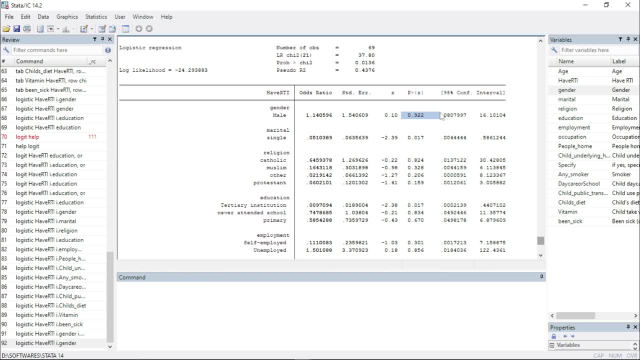 variable, so you're supposed to run multivariate analysis. marital status has now become significant. this is less than 0.05, so marital status is literally significant to having to a child having a respected tract infection. but let's see how about at if we are done. 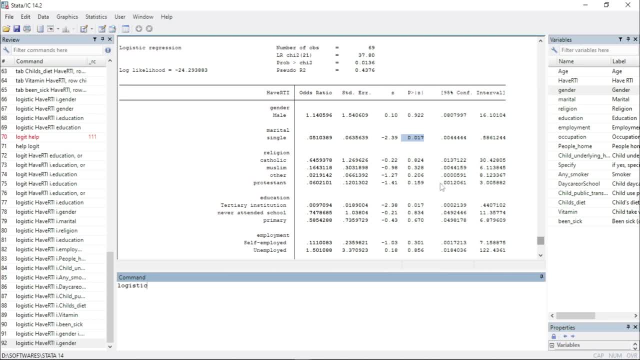 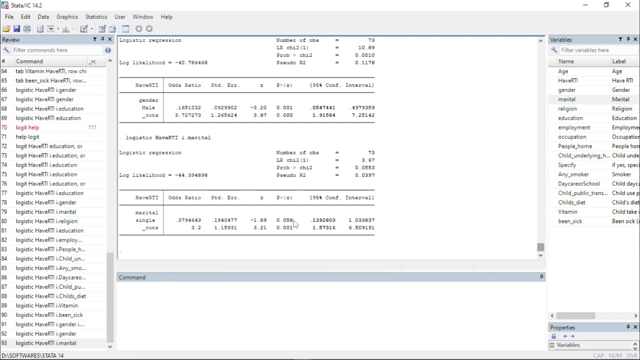 on the outer bivariate, would it be significant? let's see logistic and then we have um that matris status and then i put here: all right, look at that, it's not 0.058, this is greater 0.05. so my total status at bivariate is not. 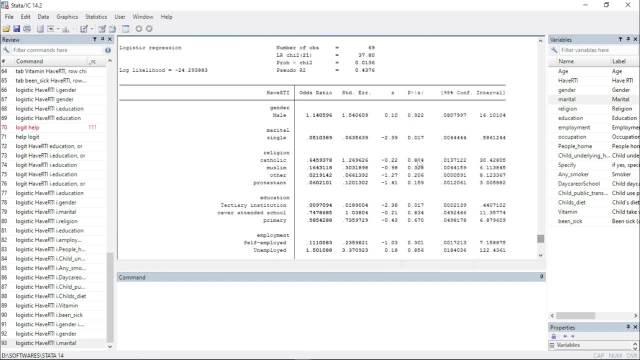 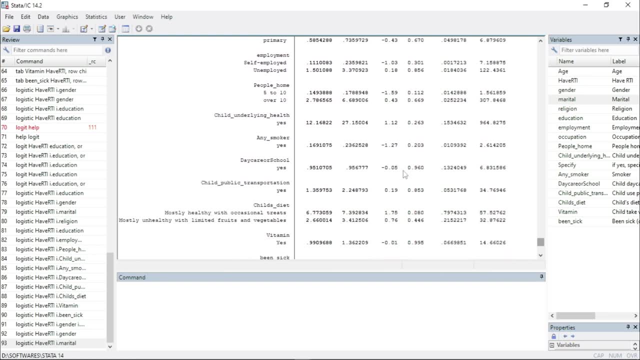 significant, yet at malvern is significant, so this is a true significant. so So that is what I did on this analysis, So this is what I've performed now. This is everything that I've done within this analysis and it has come to the end. 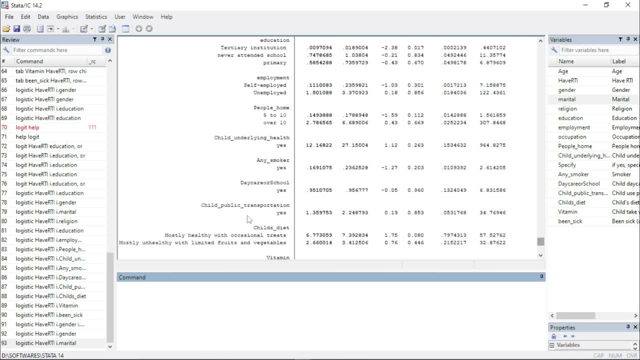 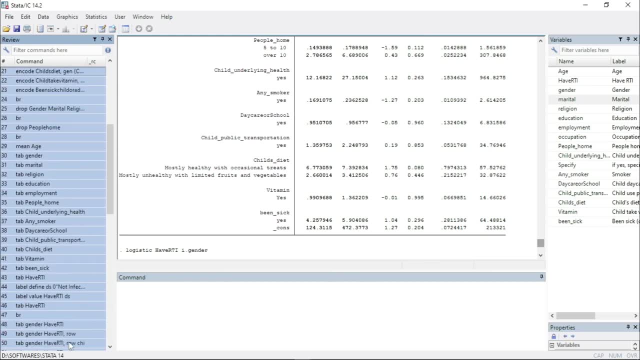 So the client wants the output. So, lastly, what do I do? One, I keep all the records for the commands I've run in a do file. So I copy all the commands I have, open a do file and then save all the commands I've been running. 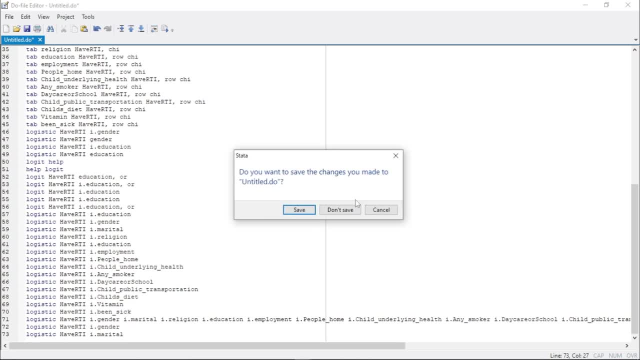 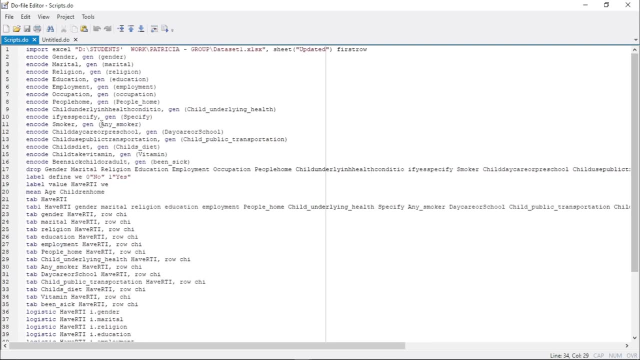 will appear there. then I edit That one. I keep it just for future use Now. so it is well saved somewhere. It's where I was picking some of the commands from, So you keep all the commands you have run in a do file. 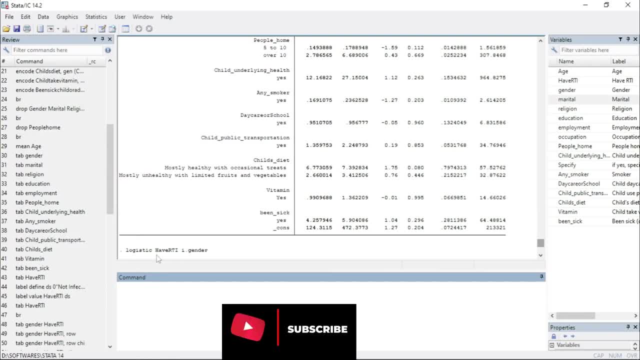 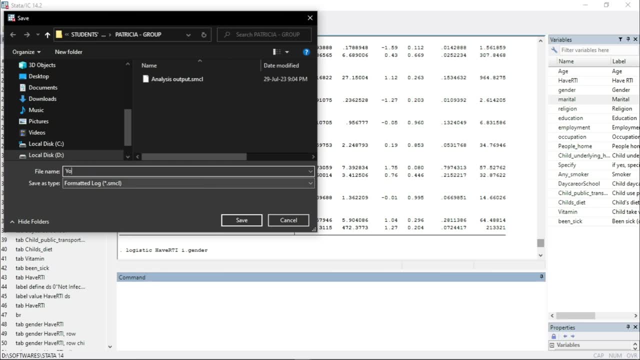 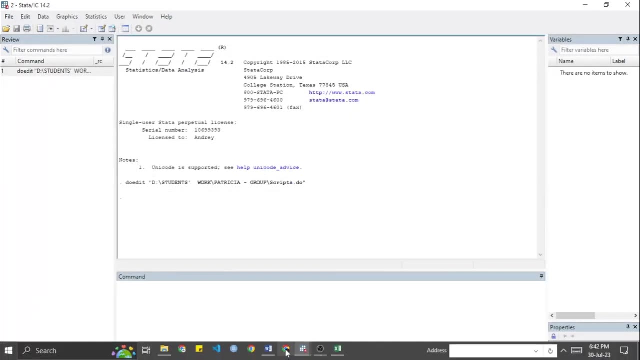 Then next, if the client then wants me to give them the output, and then they write the write up, I just come here, open a log file, begin a log file, Then I say your analysis, For example, and then I need to run the analysis. 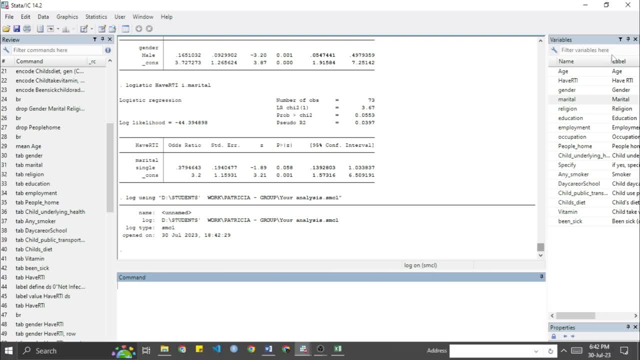 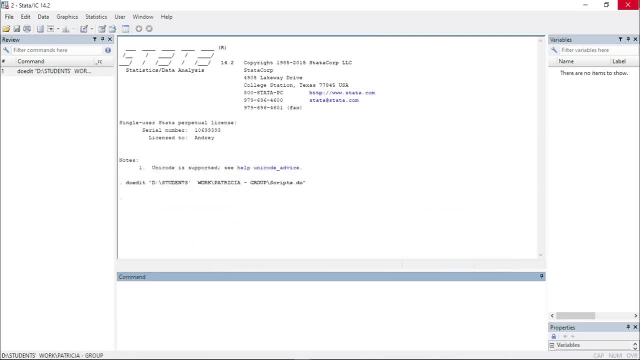 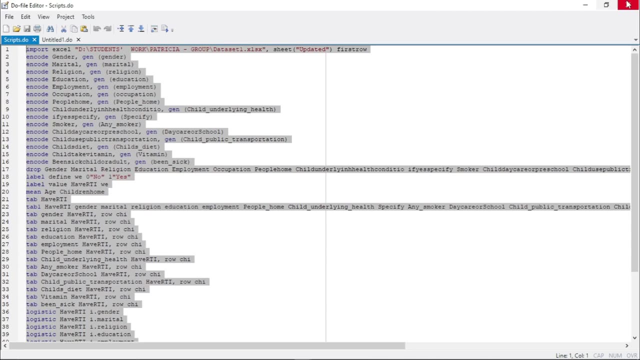 of course, for me to be having that output available. So, in that regard, I should be able to run all the analysis afresh. Okay, where are you? So you run all the analysis afresh. So let me just copy all these codes. 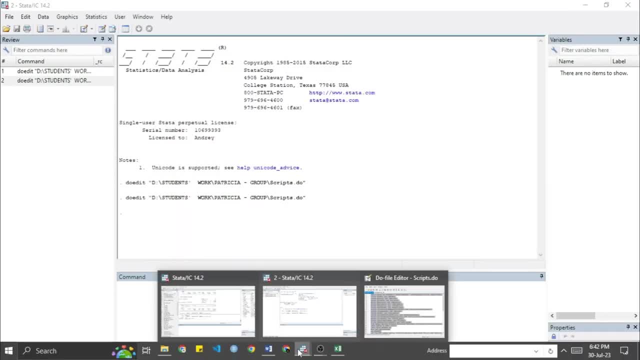 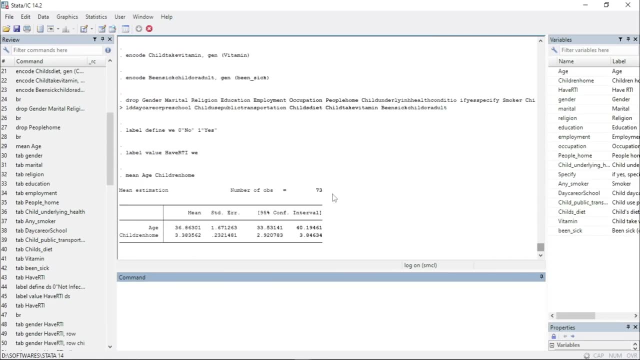 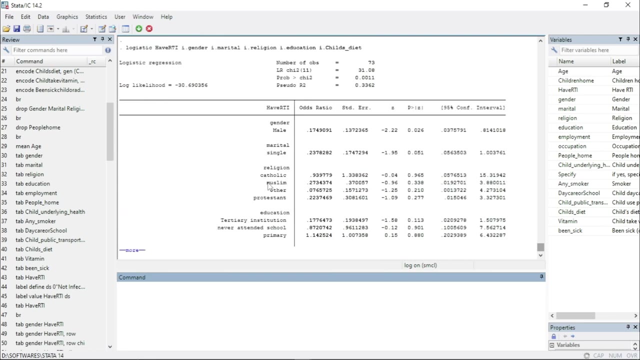 Okay then, since I've opened already my log file, so you just run all that and then it will run for me the analysis. It will keep all these analysis because I've already kept the codes I've used. All this will be automated. 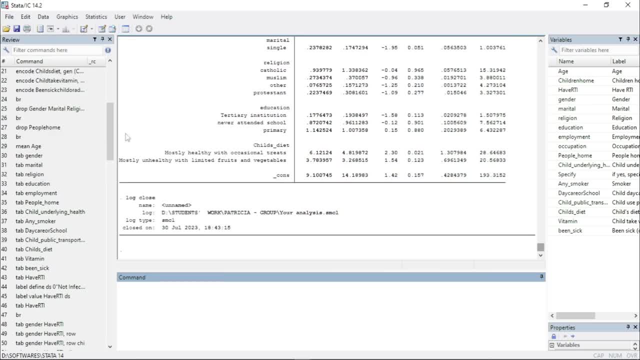 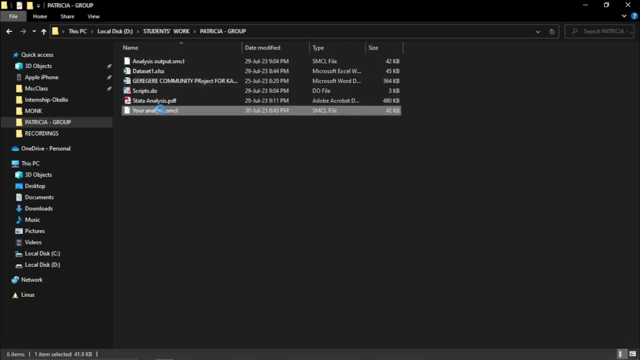 So I can now come and I close off my log file And if I go to where the log file is being kept, so it is here. your analysis it's there If you open it, if you happen to open it with a starter. 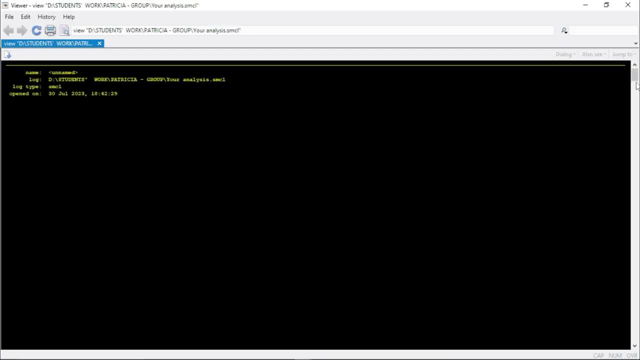 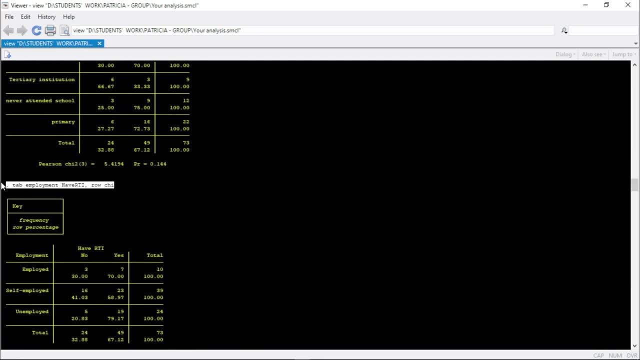 it should be able then to give me all the output Now, this I will then share it with the client. It has all the output for whatever I've been running. Codes are hidden, all that. This is a black, a black screen. 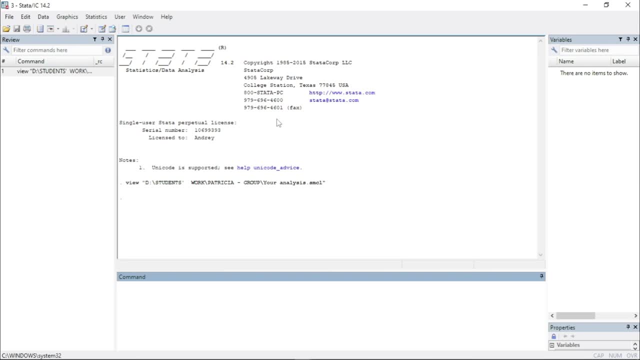 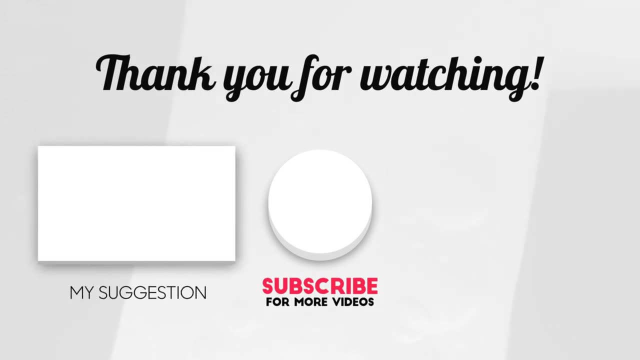 So this is what I'll share with the client And with that I'll be done with the analysis using starter. The client is happy, Everyone is happy, and I'm convinced. So thank you so much and see you next time. Make sure you can follow up, apply it in your study and you'll be good to go. Thank you.